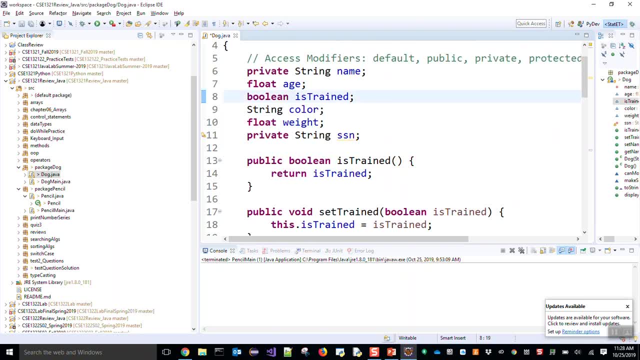 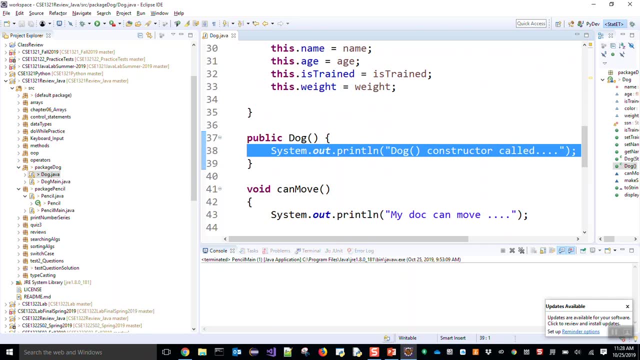 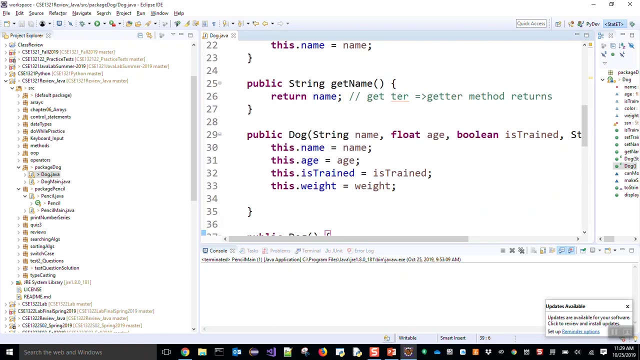 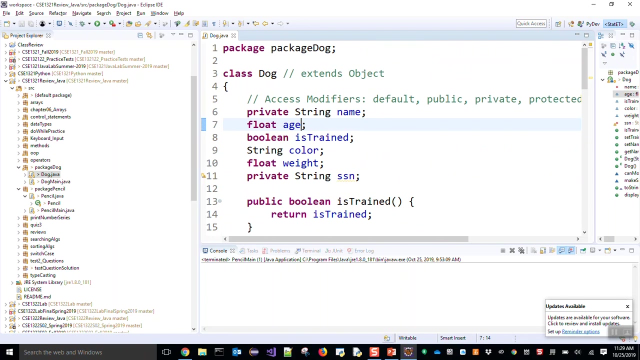 By the way, let us review, what is a constructor? A constructor is a method of a class that has exactly same name of its name, right? Constructor is used to construct or to assign values to the fields, to the class field for each of the individual objects, when you create an object we call the constructor. 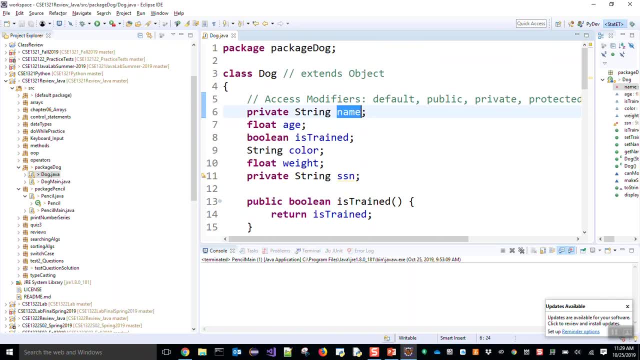 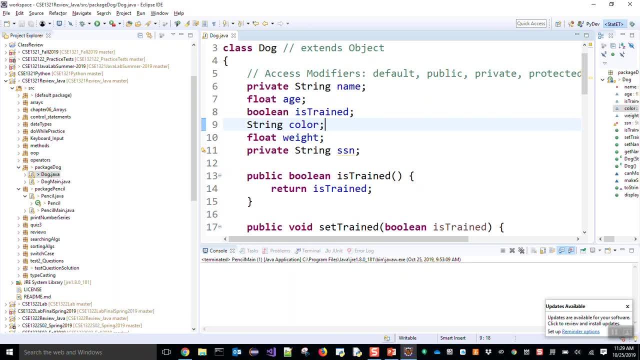 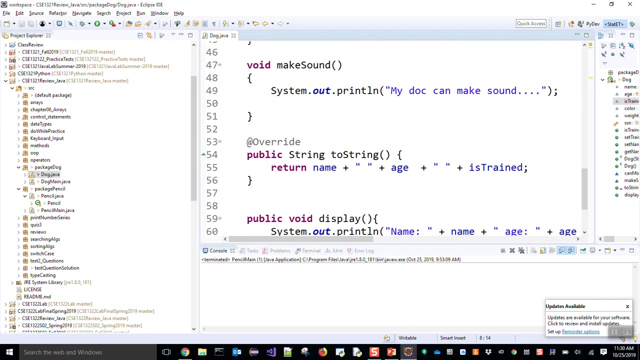 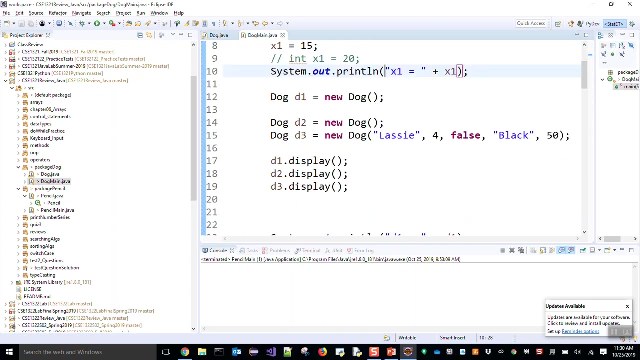 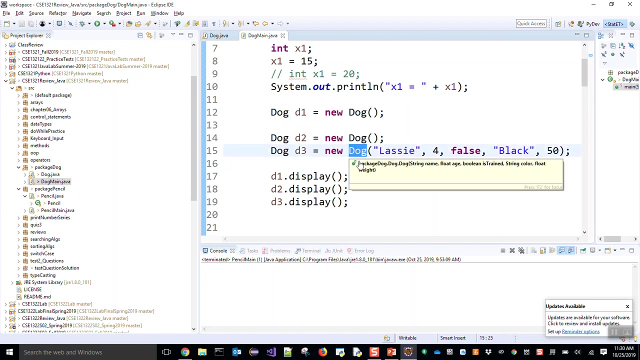 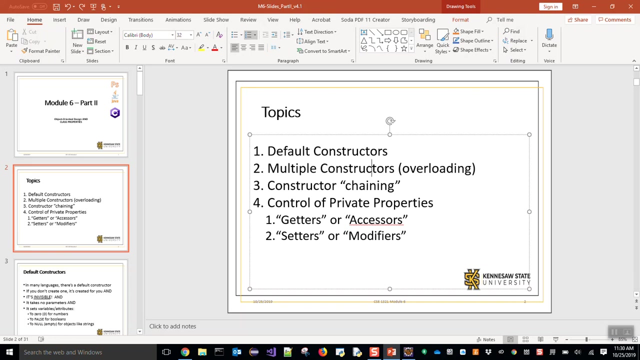 this point you should understand the difference between a class and an object if you would understand the difference between a class and object okay a class contains some variables or fields when we declare an object for each of the individual object we have some individual values for each of this field by doing so we are defining a complex or compound data type so when we create an instance of a class we create the instance that has that contains values against each of this field okay a constructor is used to have to assign values taking these values so usually when where do we call this constructor we call this constructor within our main method or driver method in order to in order to create when you create a constructor and object we use this we call this color structure okay so this is a class this is default constructor is calling and this is calling an augmented constructor and we discuss that a class can have multiple constructors this concept is called method overloading okay in term when a class contains multiple constructors the method must be different in terms of parameter type or number of parameters okay sometimes I can have two parameters in one constructor and another constructor 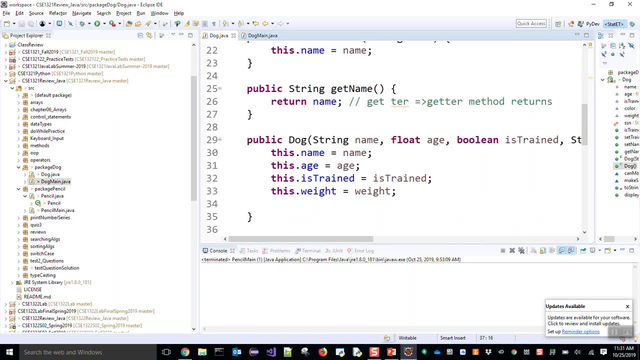 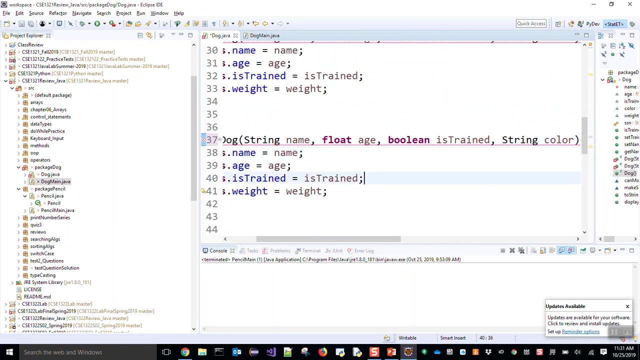 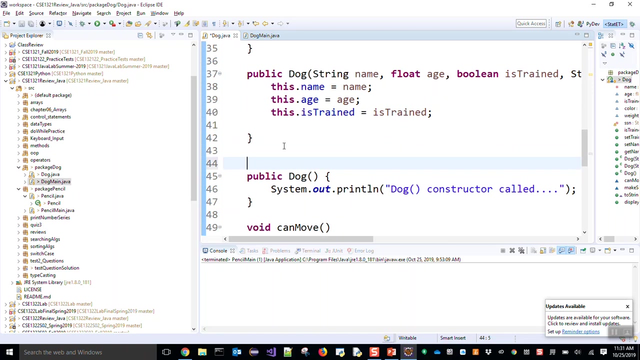 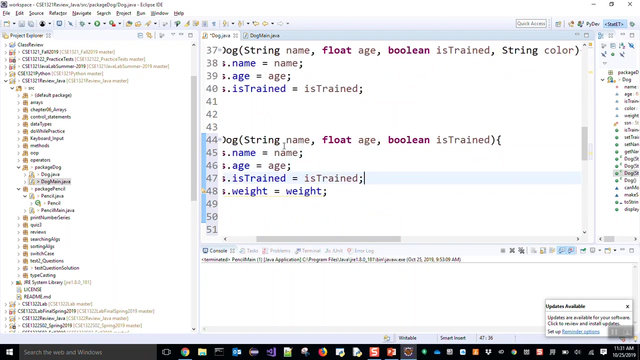 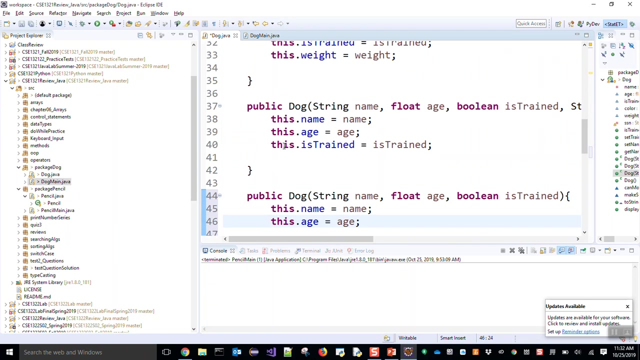 this constructor does not have any parameter but this constructor has one two three four parameters maybe and you can have another constructor name like dog with three constructor that will work but if you give exactly same number of constructors it will not work you say this is giving an error so maybe you can have another constructor without weight so then if you say I don't need weight so then it is good so this constructor has three arguments and this has four arguments and this has no arguments and maybe I have I may have another constructor that will have two arguments okay this is good and this is good as long as these constructors have different numbers of constructors it has three by default although these are same but three you may have number if number is same the type will be different type needs to be different okay either this difference will come in terms of either number of parameters 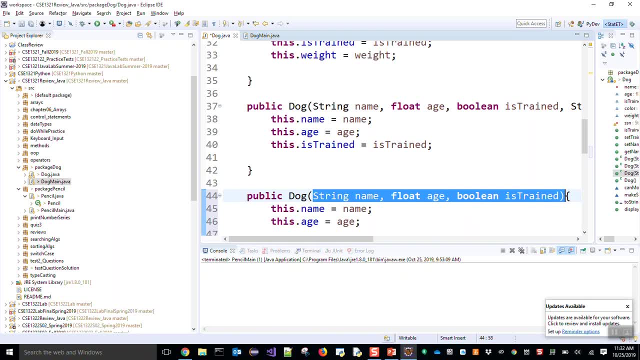 that means two or three or four or type for instance this has all same type so 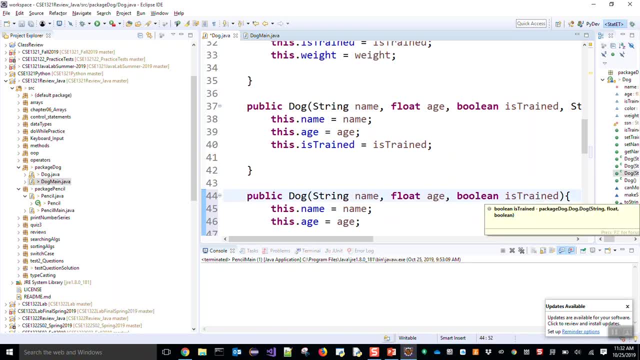 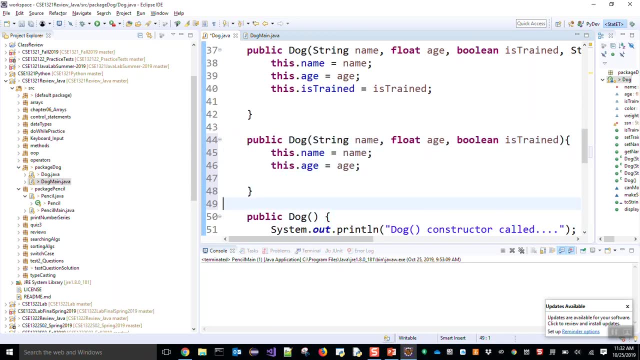 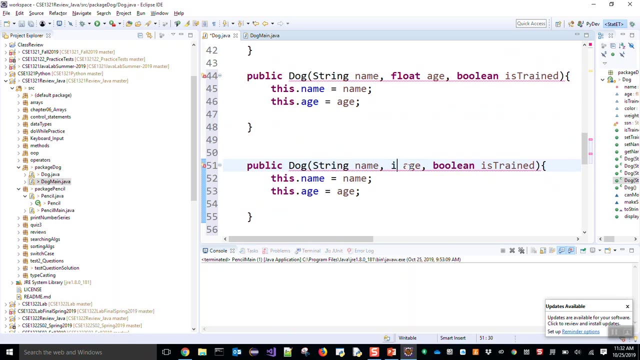 its name name age and boolean test in time so I cannot have another parameter for instance like you cannot have another one like exactly same type this will make an error but you can have for instance maybe is you can have integer if you say age is integer over here so you see that these are numbers of parameters are same how many numbers three right and here are also three but the difference is tiny difference what is the difference here it is age is integer type and here is this fluid type so it is permissible okay but you cannot have same type for instance you cannot have integer type you cannot have it okay so based on the value pass actual parameter value for the actual parameter you pass when you call the constructor it will call the appropriate one whether if you provide an integer value for age then it will call this one if you provide an a fluid value a decimal value for age okay so this concept is called method our learning okay the class have 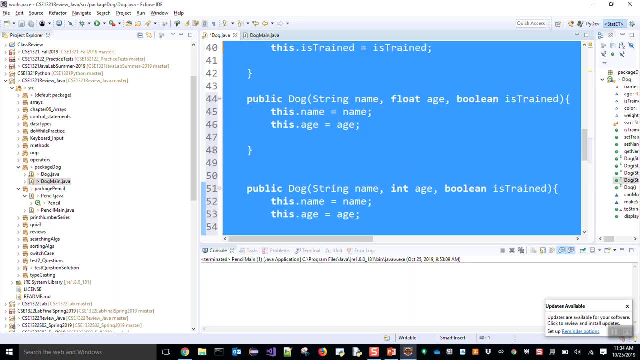 multiple methods but these methods must be different in terms of their parameter 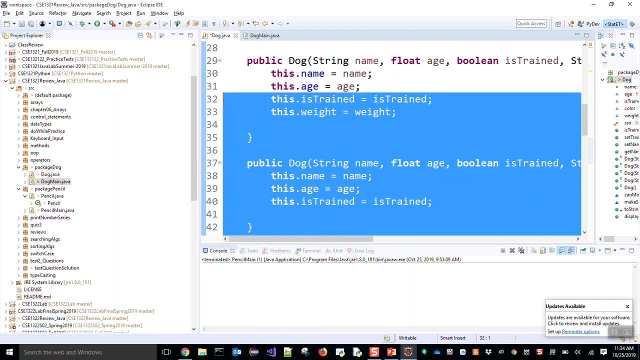 name or number of parameters so everybody understand method of our 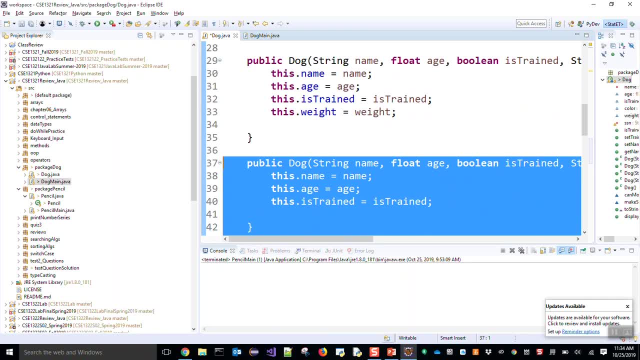 loading so constructor is a method so it can be overloaded 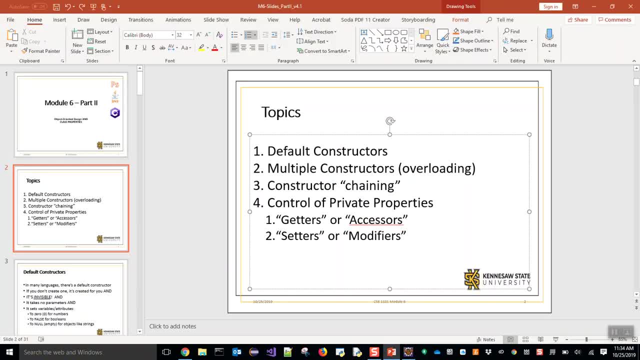 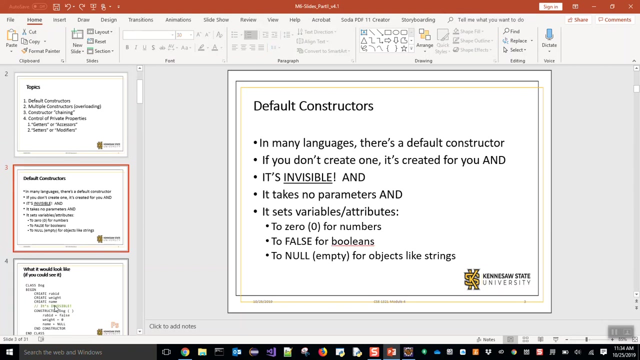 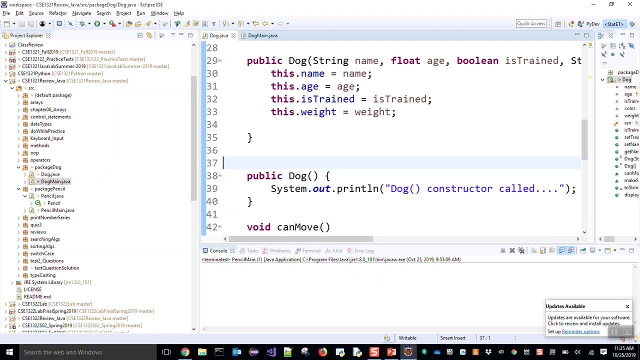 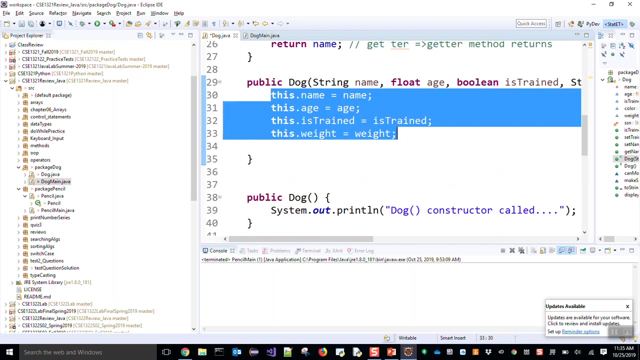 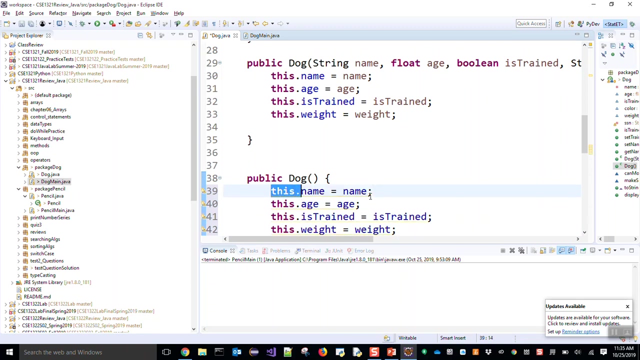 okay we discuss this and okay another concept is constructor chaining I will discuss this okay and then another concept is that called control of private properties of a class we do use getter and setter getter method is sometimes is called accessor or setter method sometimes called modifiers or mutators in some book or in some places you may see that mutators this is called setter method okay I will go through this so default constructor default constructor is used either say a default constructor for instance for my dog constructor if I do not have any default constructor then assume that there is a constructor like this okay but we put some message so that we understood that this default constructor is called another way there is another use of default constructor if we want to set some fixed value for our for our fields for instance if I want to say all of my dog will have name same name exactly exactly all of my dogs will have same name they see okay all of my dogs will have is maybe two years equal to two years all of my 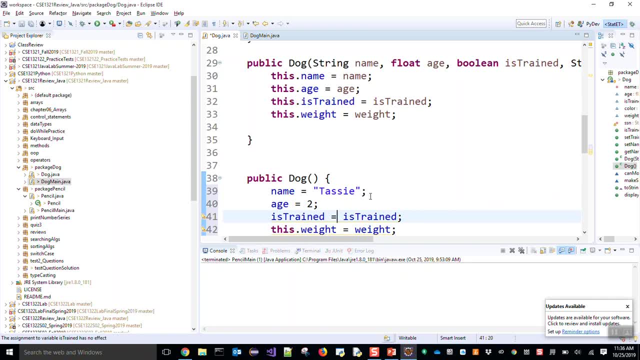 dog will be trained true and all of my dog will have weight and 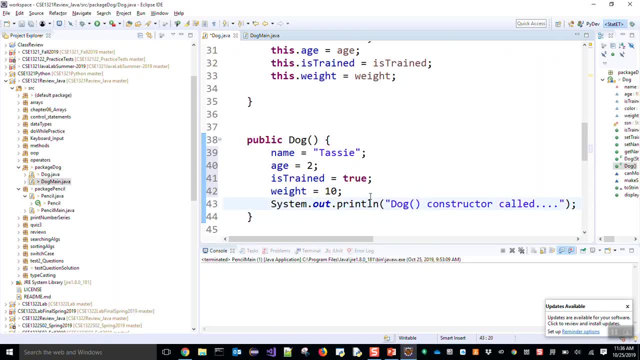 maybe ten pounds so this is called default constructor I am setting up some default values so all object will have this same value right same value so actually this is a rare case that we will use default constructor to set I don't like all object will have same attribute right same attribute the same value will not have same value for each attribute then there will be confusion for instance if all students in this class have same name same ID same age same GPA then 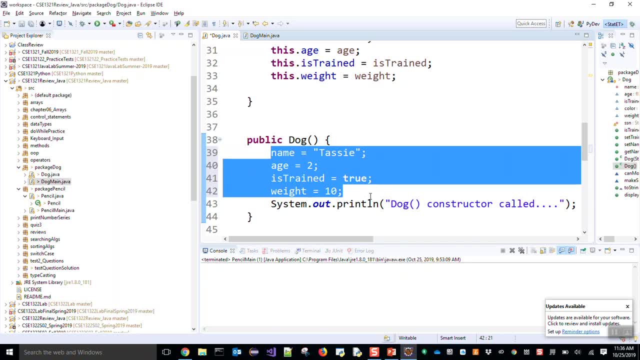 there will be confusing right in this in a real world that is not expected and that is not possible so even if I say I give an example these are two clips you must see from the back 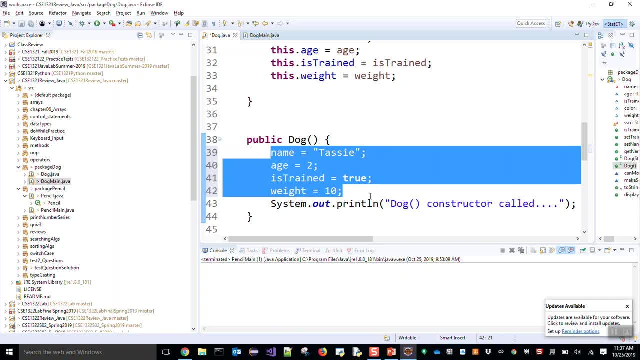 you can see so all these are same exactly same so all these are same exactly the same same brand same color same size but these are two different object we cannot say that this is single object two different right because we cannot for these two there is at least one different attribute for instance think 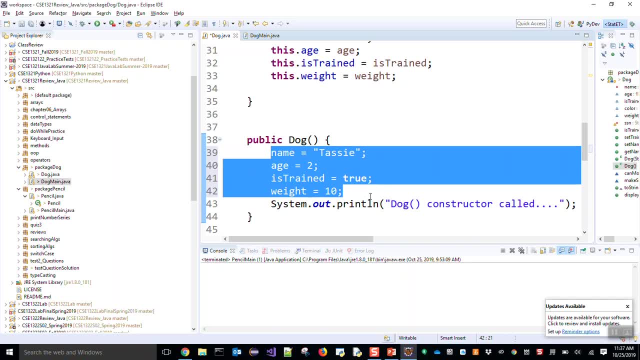 about position for every object in this world there is a position attribute right 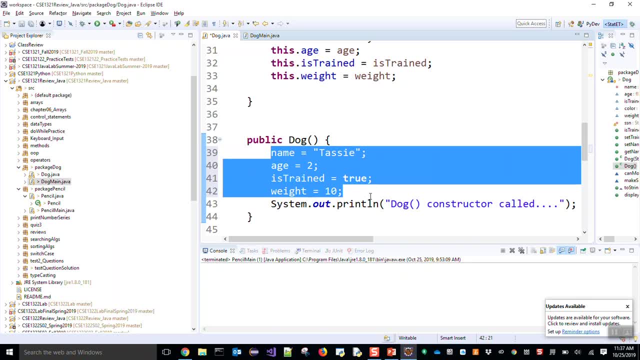 position value for these two object all these are same but we cannot have same position value 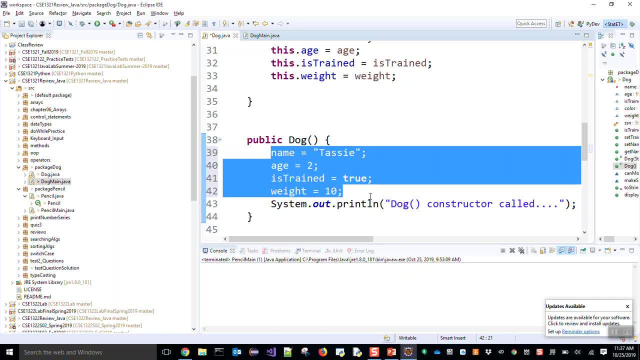 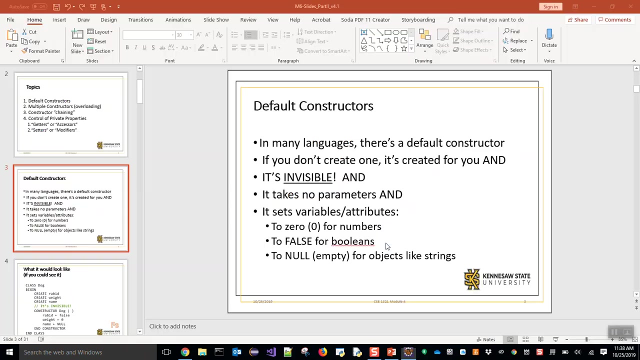 so you cannot put I can put one top of another one or bottom of another one or left or right or another one so if you can exactly have even two this alike object but these are two different right okay so by default if we do not assign value for a 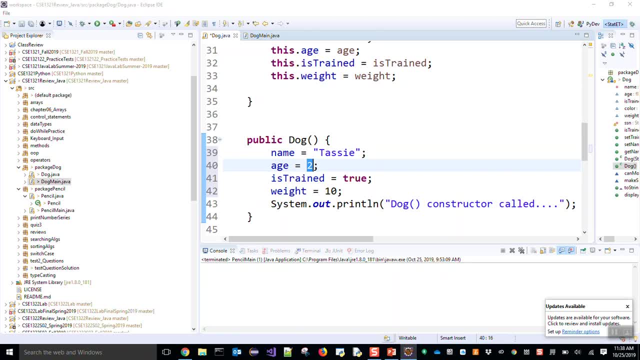 integer type we know that this in for an integer type we takes zero by default 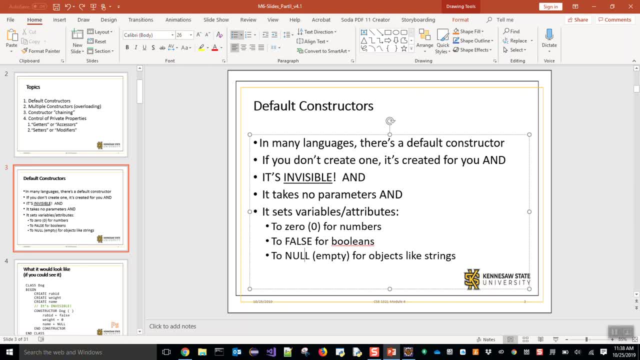 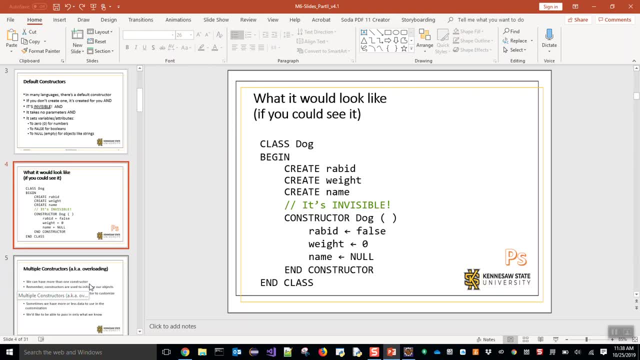 value and for boolean it takes fall and for object type it takes null okay and we discuss constructor right so if you write pseudocode then you have to write 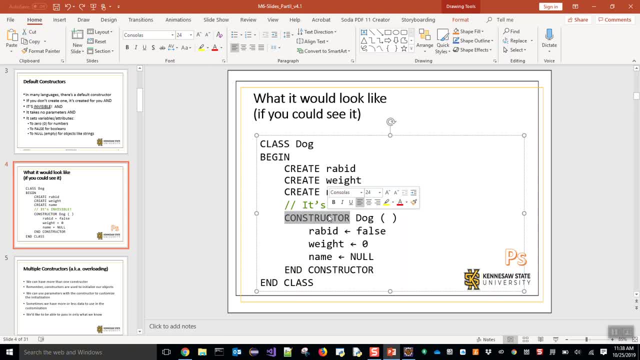 the constructor keyword okay or in uppercase and but if you write pseudocode if you write program code then we do not need 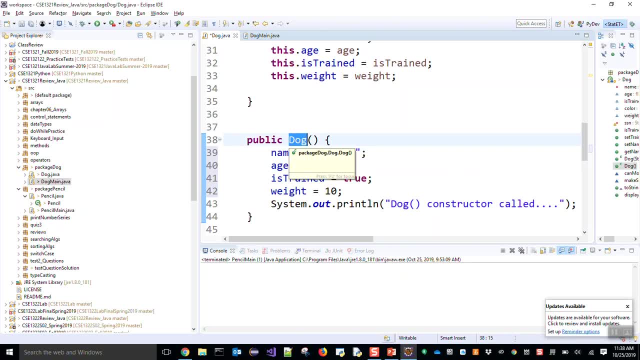 to mention that this is a constructor everybody who knows program should know who knows if object oriented program class 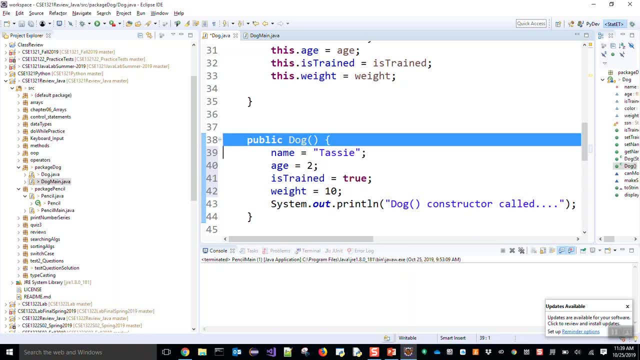 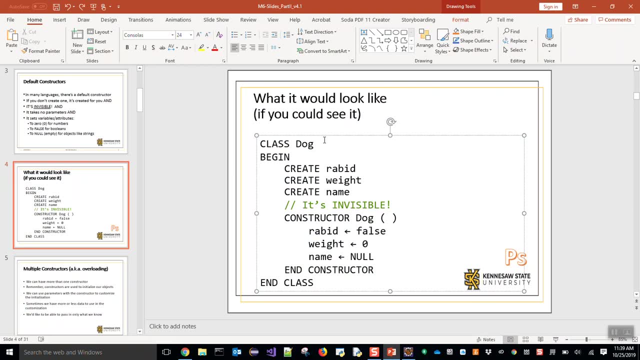 and object should know that this is this is a constructor but if you write pseudocode I encourage everybody to start writing program and practice program 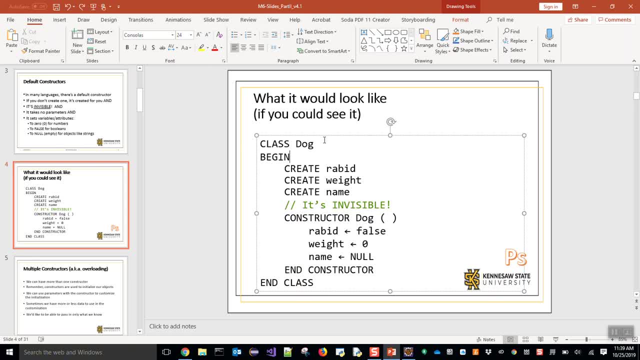 okay so if you write pseudocode then be careful you see that you have begin and we have to use the word begin and you have to use the word in in class that means class doc begins over here so you can say even that means class doc begins here okay and for create for every field we say create and for constructor we need to use constructor and you have to use a constructor to me it is a there are a lot of things to write but writing a class is easy 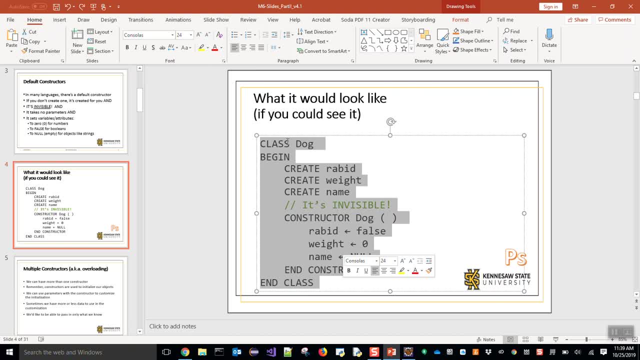 only a few lines of these all right compared to writing as suitable so this is why I discourage writing pseudocode in writing a class in pseudocode format okay 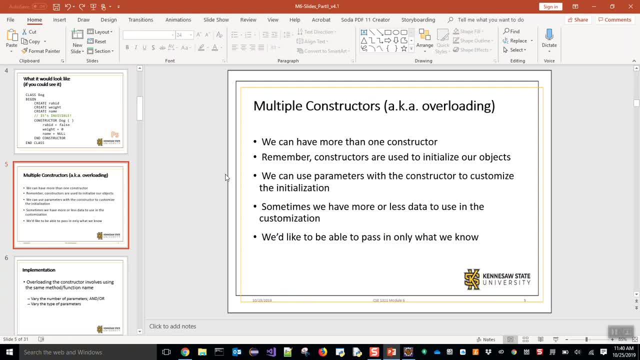 we discuss multiple constructors that is called overloading method overloading is 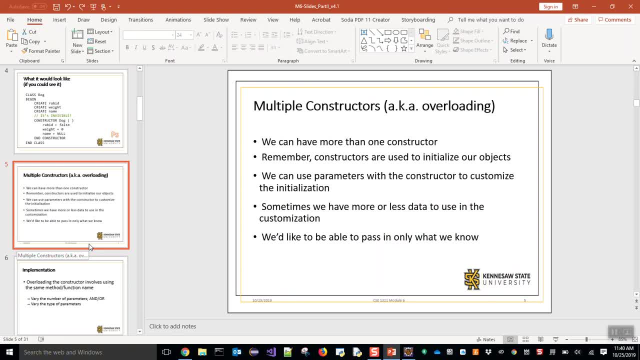 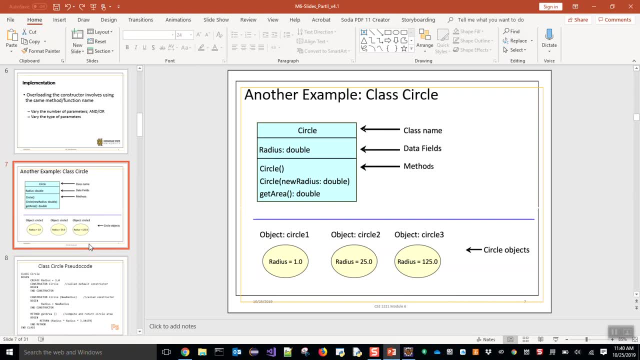 one of the important other important feature of object-oriented programming here we discuss this and this is an example there is another example of circle class circle class a circle has like in order to be a circle it needs to only one attribute should be fine radius you could give more attributes like location x coordinate y coordinate but radius is fine and if you have a circle then you can have a circle constructor or you can have default construct or you 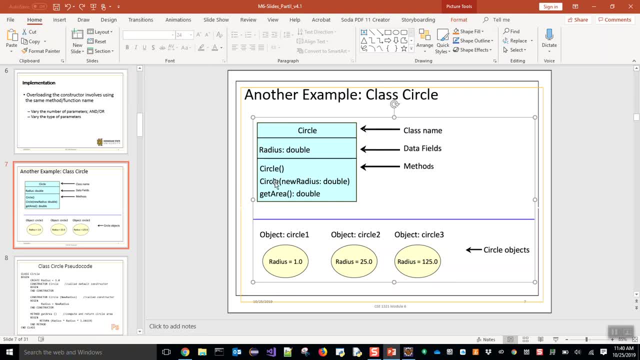 can have augmented constructor that will take the radius then you will have one method that is called gate area for a circle we can get area okay and if we use this second constructor then we can provide any radius we want for instance we can provide it is equal to 1 or 25 or 125 or 2 or whatever value we need success 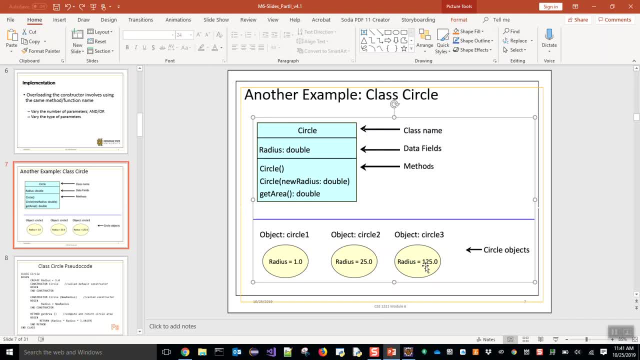 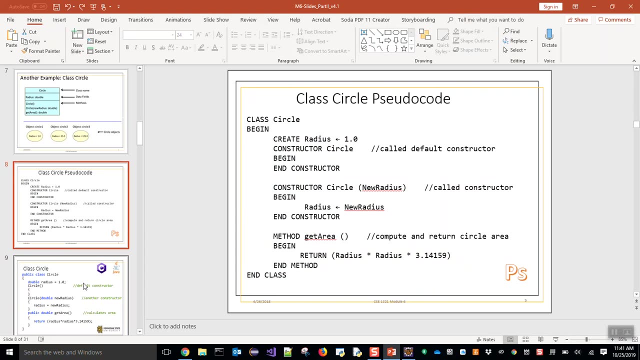 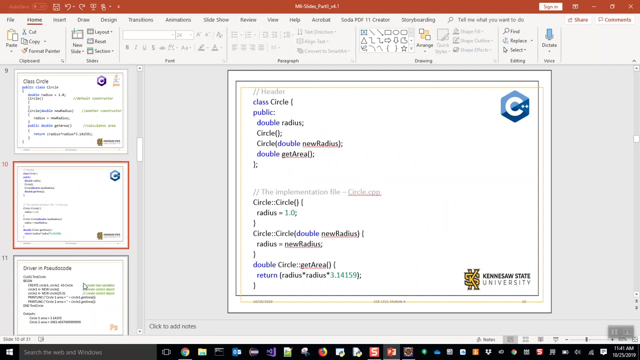 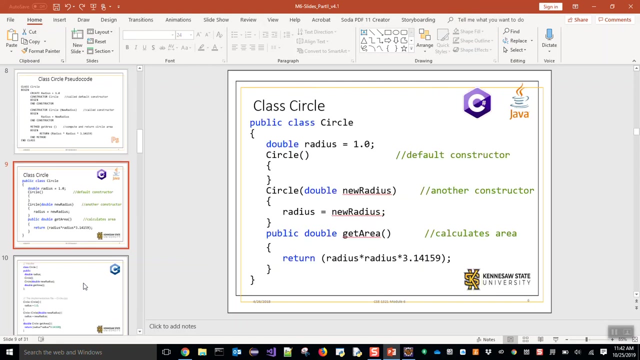 circle is my class name and radius is my data field and these are my methods constructors and other two others okay so I like everybody to practice programming this circle class okay we have our pseudo code over here and we have Java program code over here and we have C sharp C++ code over here do I have C sharp okay okay it has C sharp also so so it doesn't have Java okay it has Java for Java and C sharp it's almost same okay so this since there is no print method over here so Java infrastructure is same exactly okay and another thing that 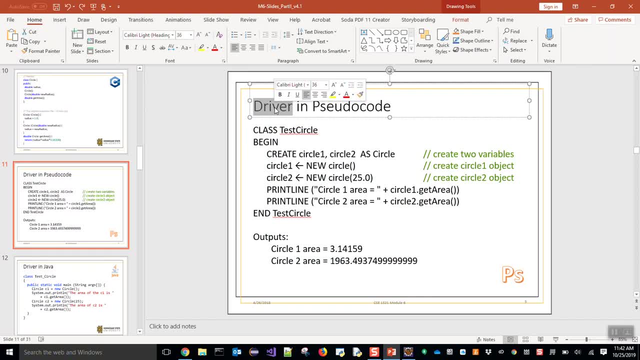 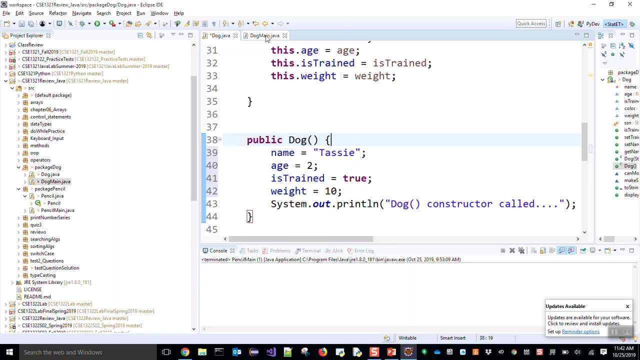 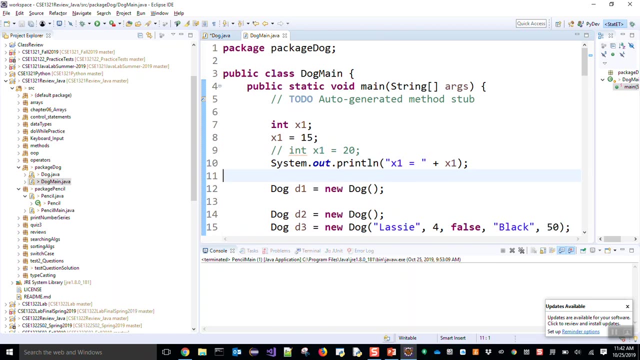 a driver uh driver in procedure sometime we call this the method of the method that is used to create constant object that is called main method or driver method and the class that contains the main method is called main class or driver class so here I gave name drug name some people may say 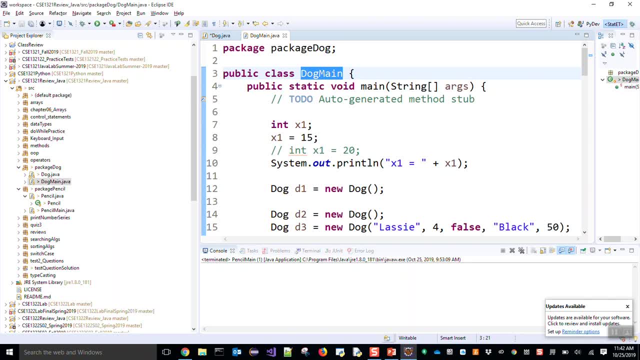 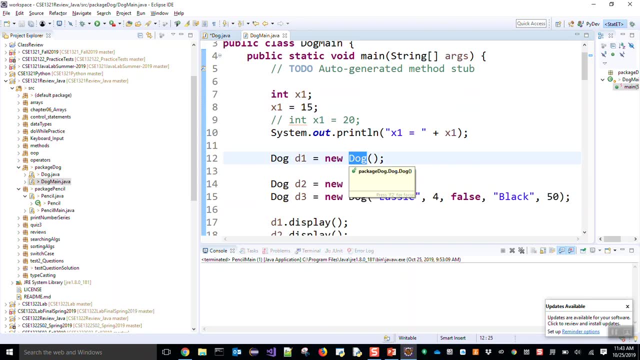 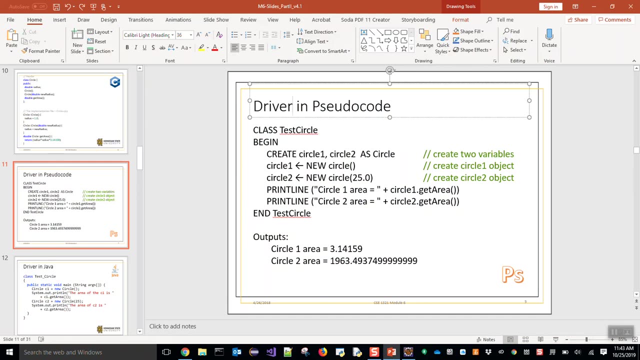 drug driver this class name okay and because it contains the main method that is being used to create dog distance okay so you may hear sometimes it's a driver driver method okay or main method 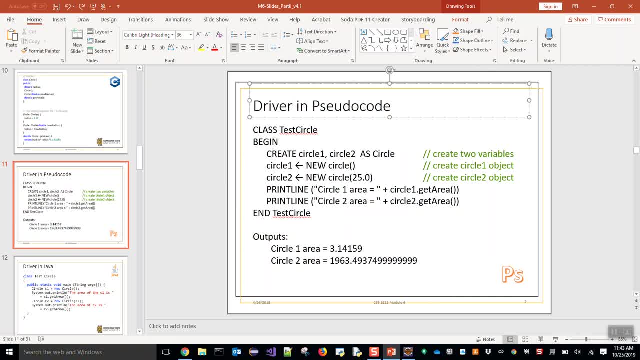 driver class or main class okay the class that contains the main method is called main class or driver class 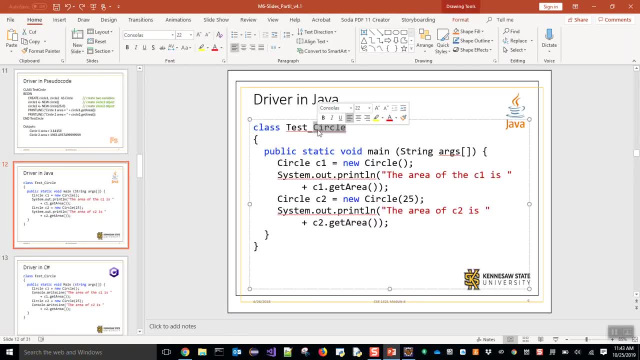 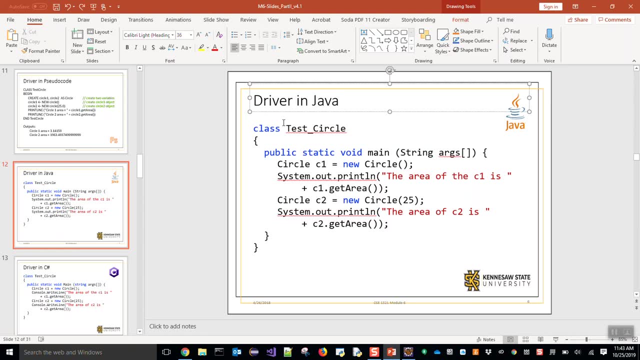 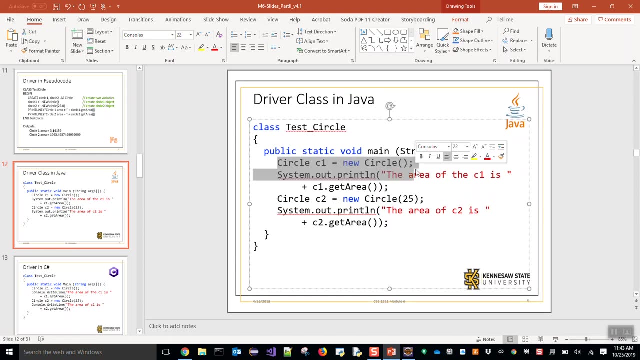 so here my test circle it contains my main method so my test circle I would say that this is my driver class okay so what does it do it creates a constructor circle constructor and it display the 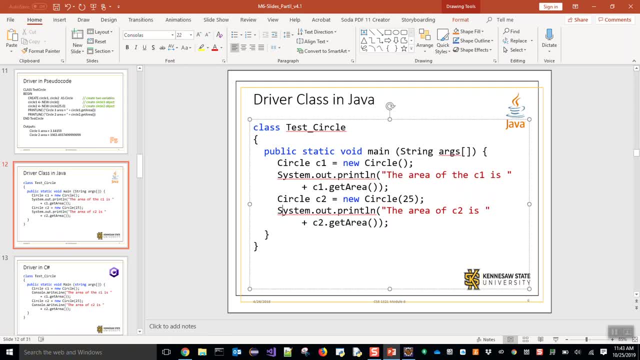 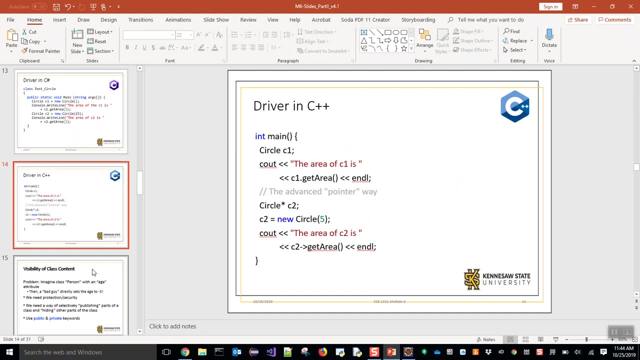 area and it here's another circle and display this that circles area that's it in java format and we have code in c sharp and we also code in c plus plus so c plus plus people know that we use 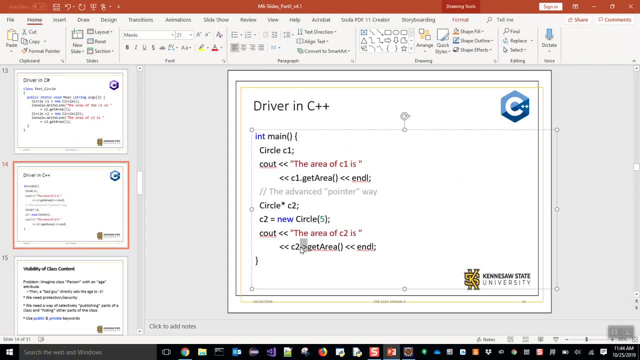 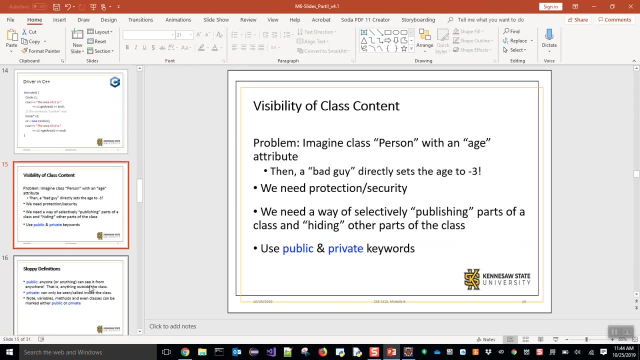 instead of dot operator we use error sign right c plus people know it okay another thing that we discussed the visibility or accessibility mode 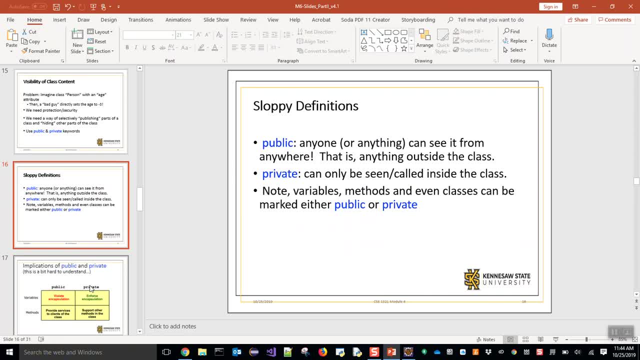 okay so visibility or accessibility mode there are actually three or three kinds 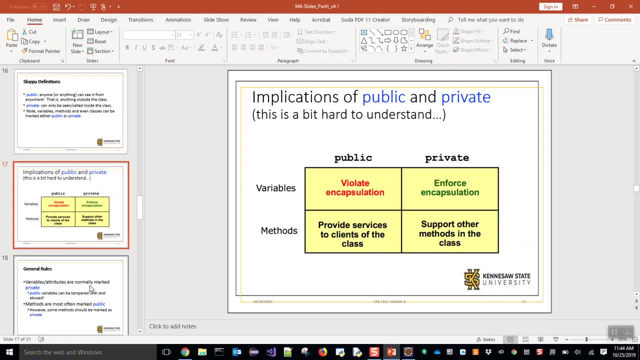 of accessibility mode in c sharp and c plus plus and java has four kind so the common type is public and private and java has also default okay and there is 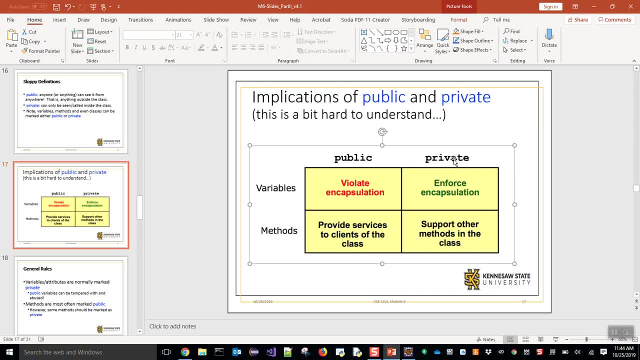 another type protected we will discuss protected later when in your next course when you understand 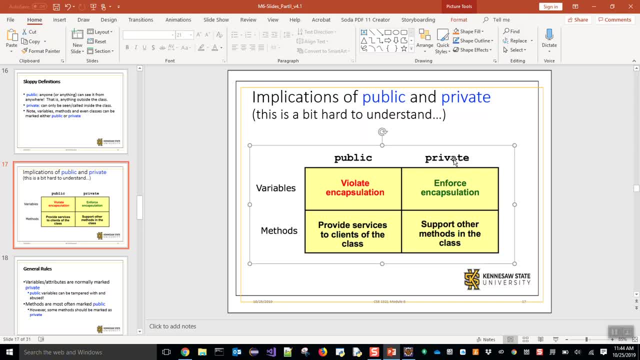 inheritance then you will understand protected protected is in between public and private so public access modifier is that a field is public that everybody can see it can use it can change 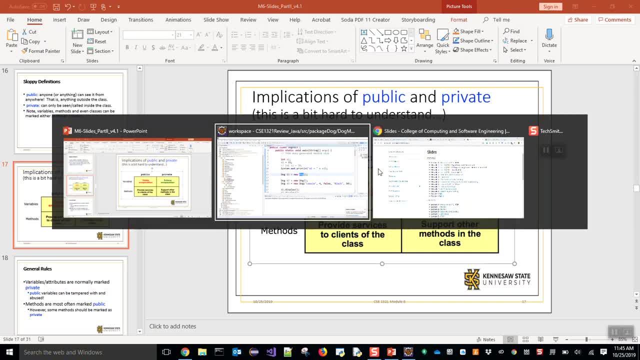 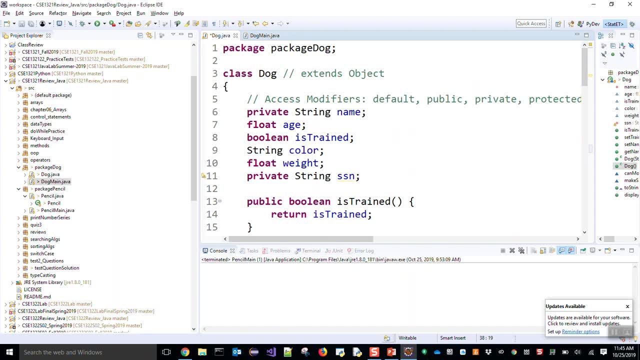 it so if I have some properties in my class permissive dot class I have some properties if I have property for instance public color 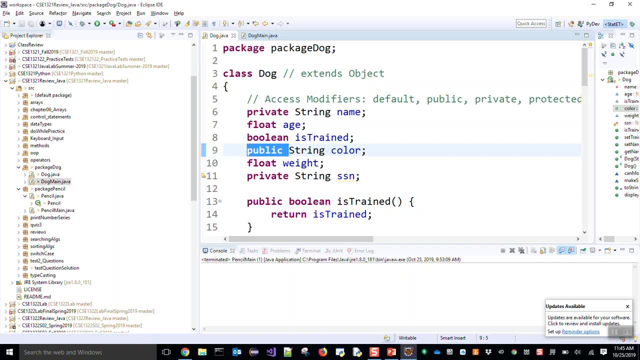 so everybody doesn't use him also right now so probably not good then these are here so everybody if this is my dog and it has public color property color color properties are bleak then a rebel I will be able to see it what is the color of my dog my friends or family we will be able to see it my enemies will be able to see everybody okay so that 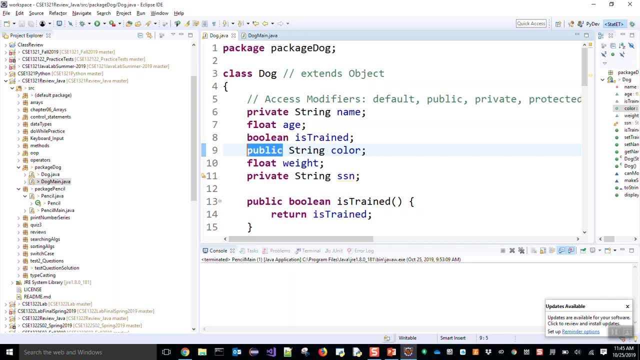 okay so for some fields or some reason we like to make some fields probably for instance everybody likes to to like to have his name or his brand probably popular right so in that case name can be 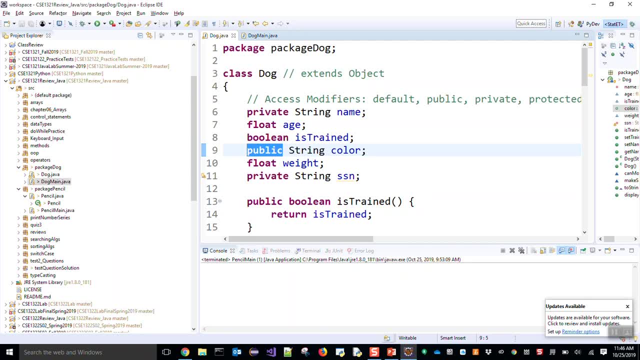 or your brand name or company name can be a public name okay but there is a risk if it is public that anybody can from outside can use it 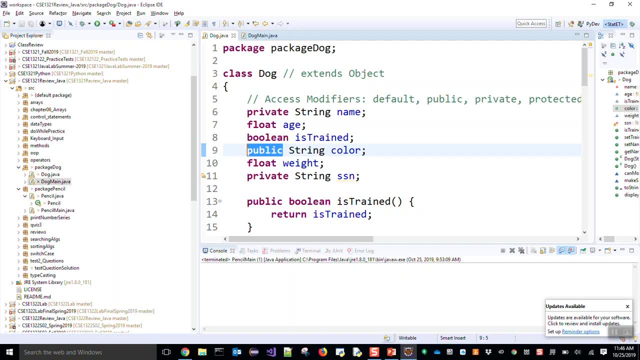 can change it maybe if it has a construct you can change it anybody okay 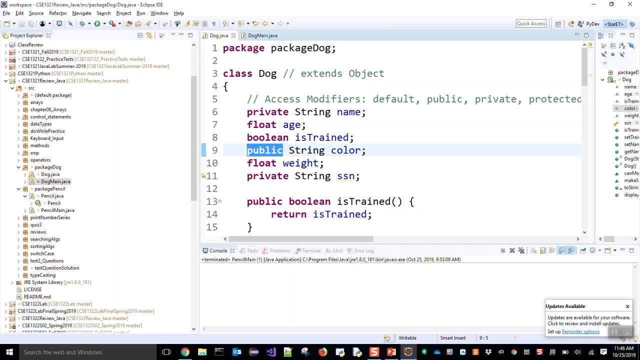 so for public property there are advantages but there are disadvantages also 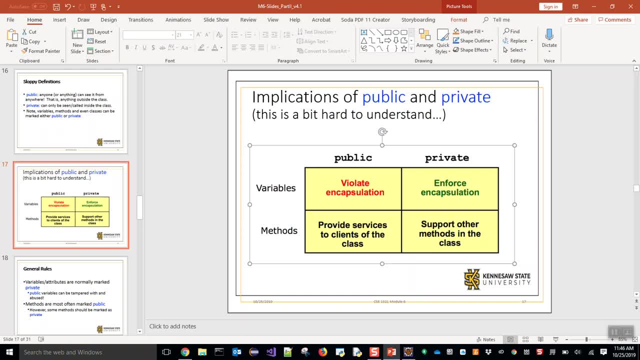 okay sometimes we do not like that my property or something we like to hide or keep in secret so that nobody can 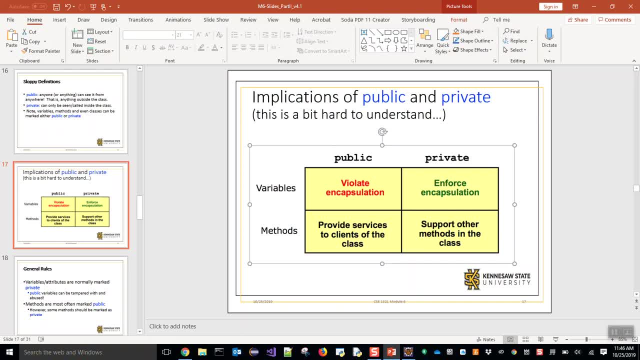 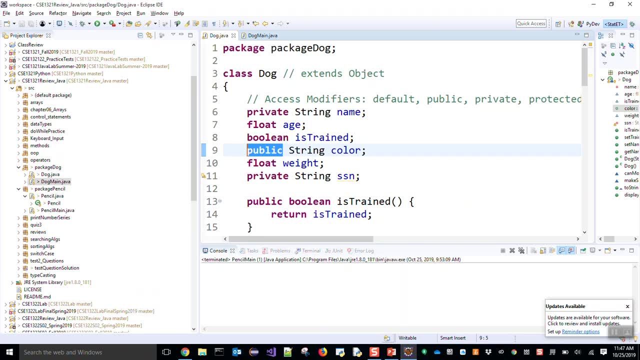 know it without my permission so if we want that someone will need my permission to see my dog name 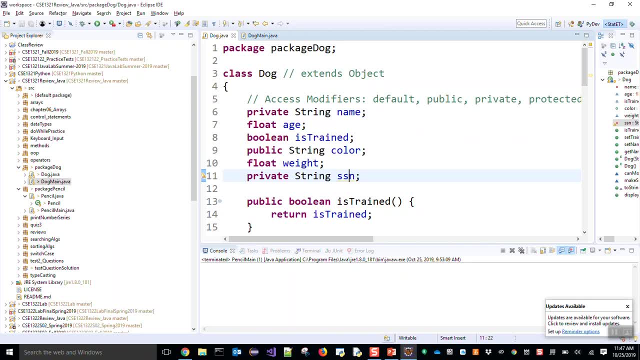 or see my dog social security number although for dog we do not have social security number but assume that may maybe have some subtracting numbers then we we saw that we used two different kinds of methods 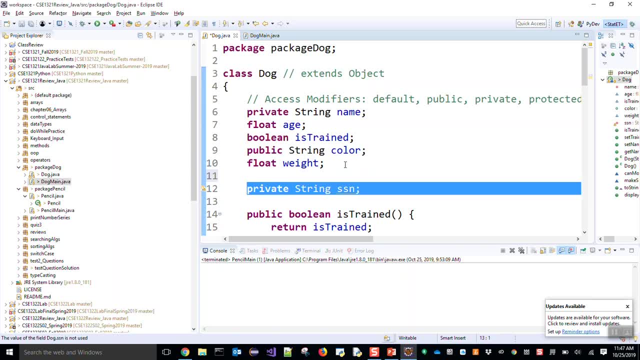 we use a secure manner to access this there are called anybody remember this what method we declared for accessing private members in our last class we discussed called yes got your note 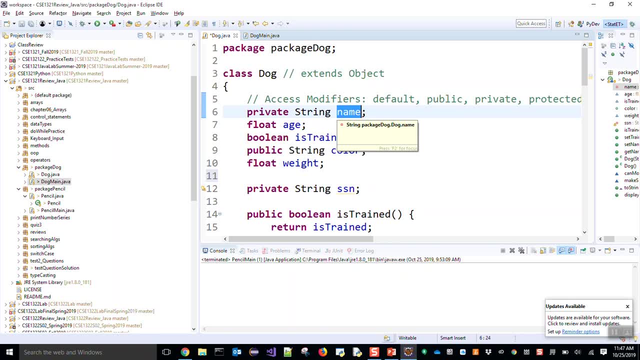 there are two methods this one is called yes setter and getters okay setter method is used to set properties for private properties if it is public then we don't need setters right 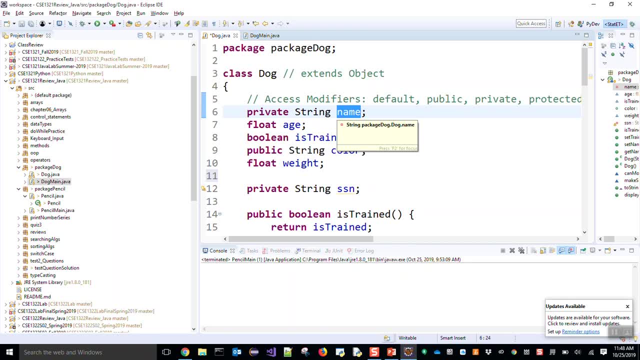 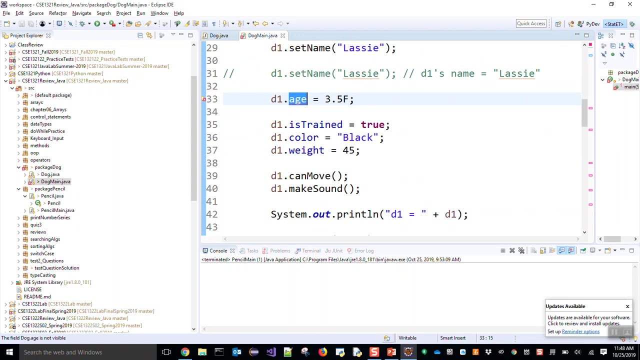 but for public also setup setter method can also set for public as well as but start matter is mainly used to set variable for public field and get our method used to get value or return value for that field right so for each private member in a field you will have one setter one line and be getter so for each public each week each private member for each private field you will have one greater and one setter okay like if I have like two if I say this one was a private if I say this one is also private so then I should have two private sorry two getters and two setters one for name one getter for name one getter for age one setter for name another setter for age you see that as soon as I made it private then there were somewhere I used directly so I'm getting an error okay 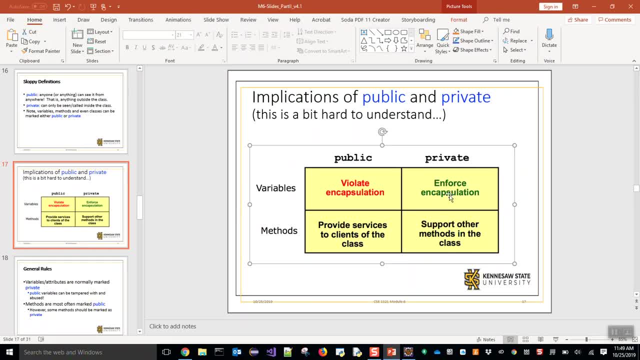 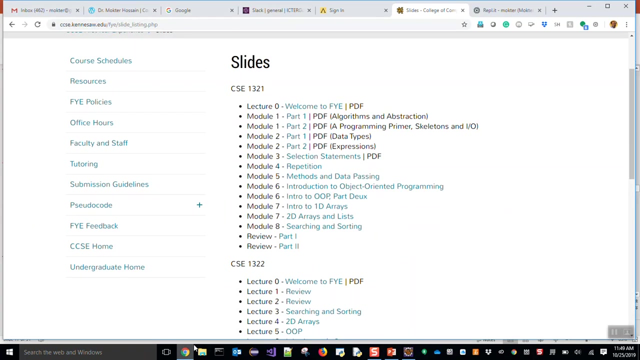 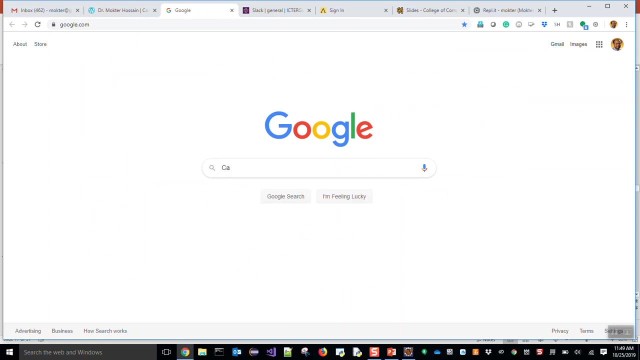 so the concept of making some field private is one of the principle of object-oriented programming object-oriented programming that principle is the為什麼 of making some field private is one of the principle of object oriented programming object oriented programming that principle is called encapsulation you may hear the word encapsulation in the word encapsulation maybe it came from from the word maybe capsule we know it's 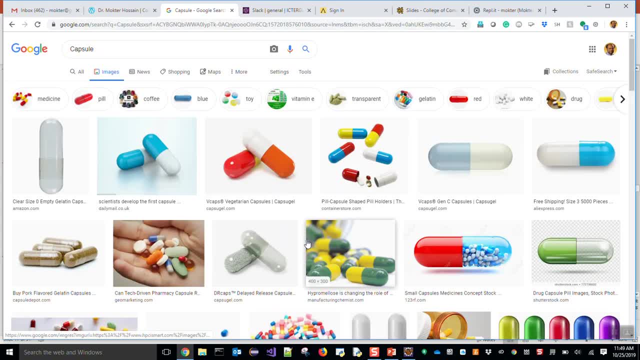 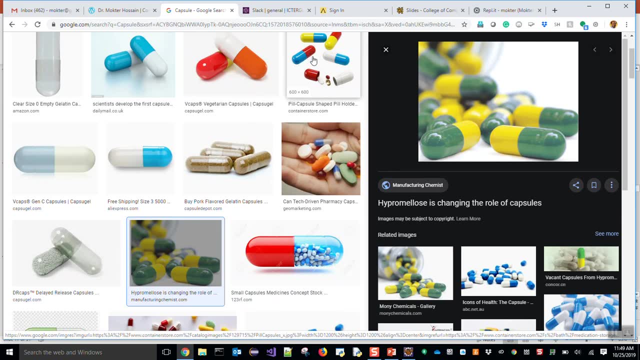 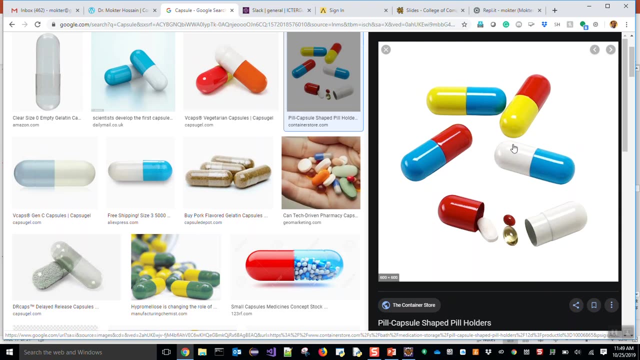 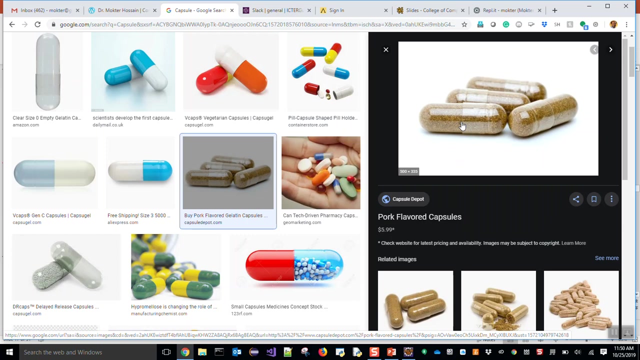 capsule is a kind of medicine that has like for instance this is a capsule right everybody knows that we use this capsule for as a medicine right okay so that actually these are the medicine there are some ingredients you see there are some some medicine inside the capsule inside the plastic a capsule is wrapped in in a capsule some medicine or some ingredient you guys will hear like a medicine something move or something something transfer something thing the relatively that is a table for the are wrapped with a plastic okay and when we eat the capsule we also we eat including the plastic right we use the capsule with the medicine the medicine are inside we eat including the plastic but as usual usually we will not eat plastic right if you if I am given a piece of plastic I should not eat it you should not eat it right and when I get it when I hit some medicine we also eat including the plastic right but you think about the situation if you buy some medicine a capsule and if you find that this capsule is leaked it's broken you will not eat it right you will not take it right you thought this is expire 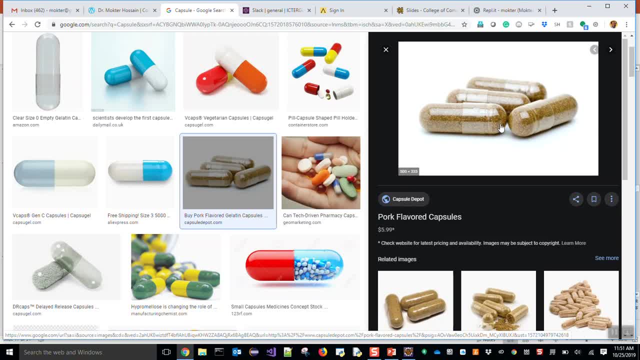 or it was used or it's not good so as long as that's plastic encapsulates is encapsulated in the capsule you should not eat it right you should not eat it 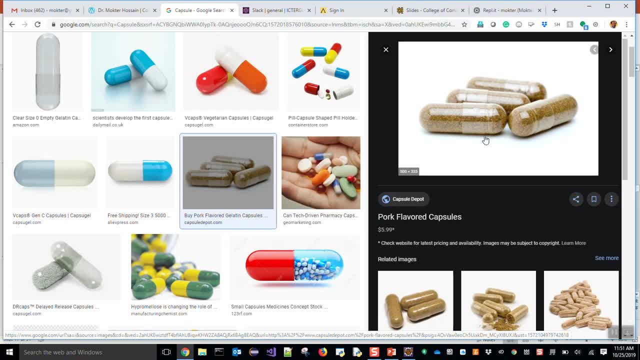 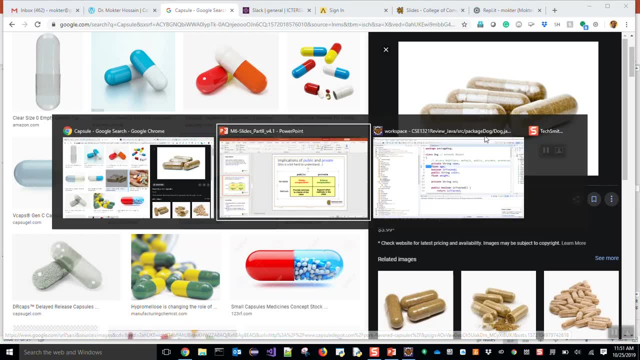 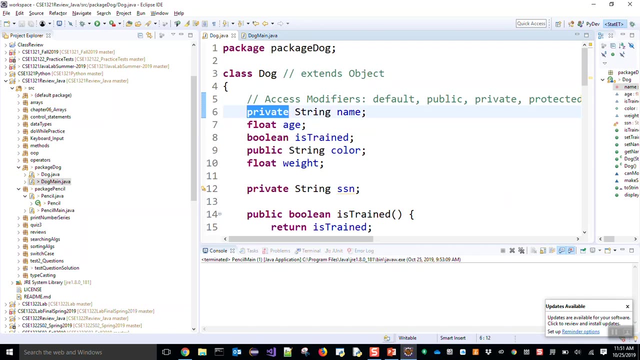 encapsulated right then we trust it we use it we believe it so same thing same thing in object-oriented programming we define some field as a private field and 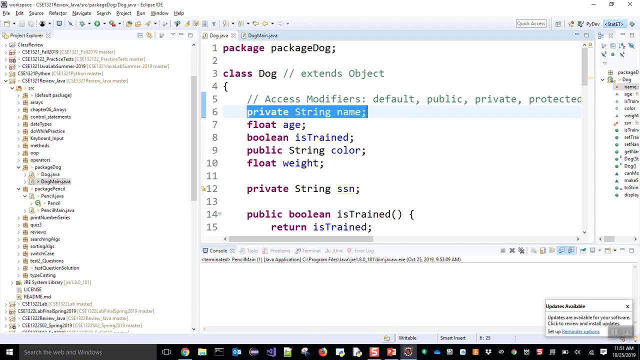 we give their accessibility or we use this using their gators and setters like 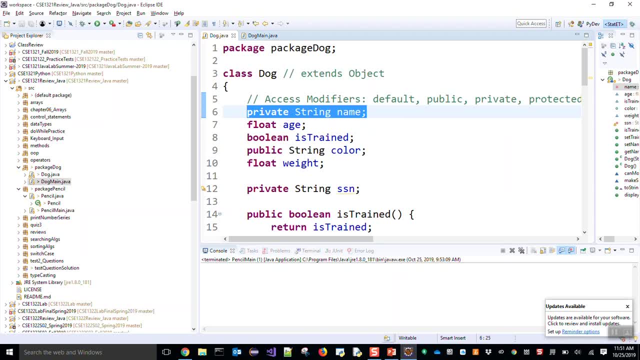 gators and setters are the plastic for the private members okay we access those private we grab these private 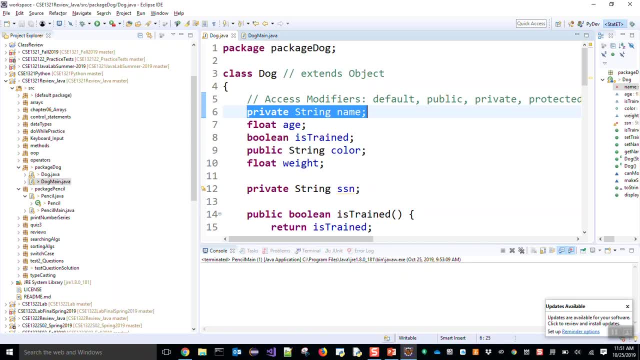 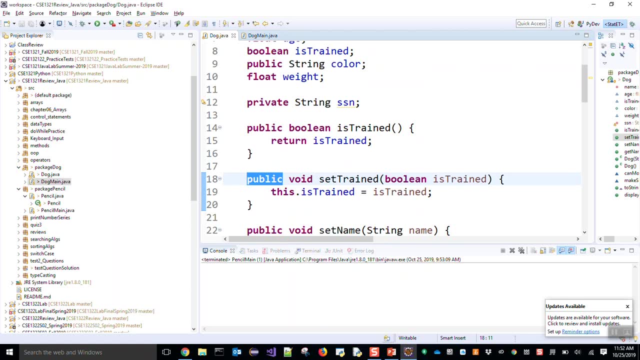 members using gators and setters usually gators and setters are public so there are some few cases that we need to make gators and setter private you will learn that later once you take advanced level programming course like software engineering course there is a concept is called singleton class there may have 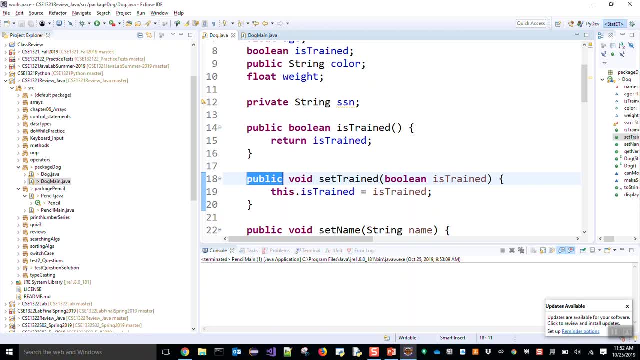 only sometime we create a class that has only one object we need to create a class then that has only one object not second object okay there is called singleton class later when you take software engineering course then you learn that so for a singleton object 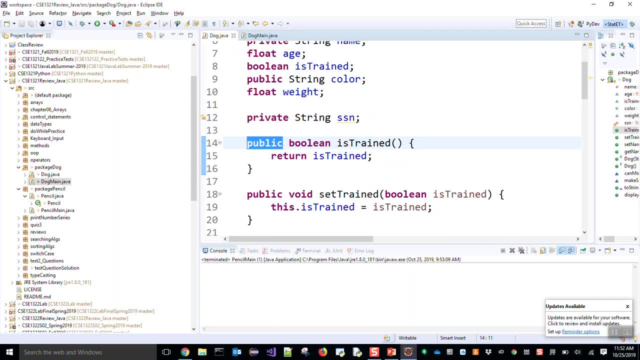 we make our setter methods as private not public but otherwise in general 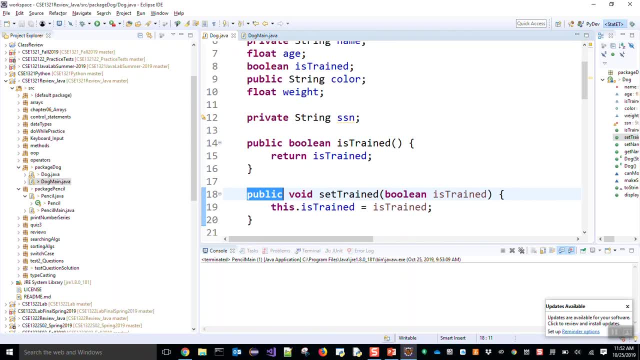 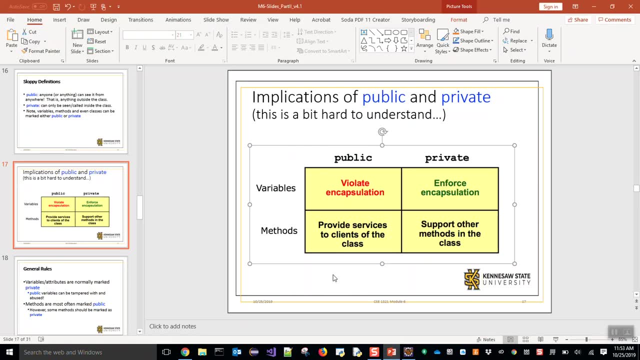 we make our setter methods and gator methods public 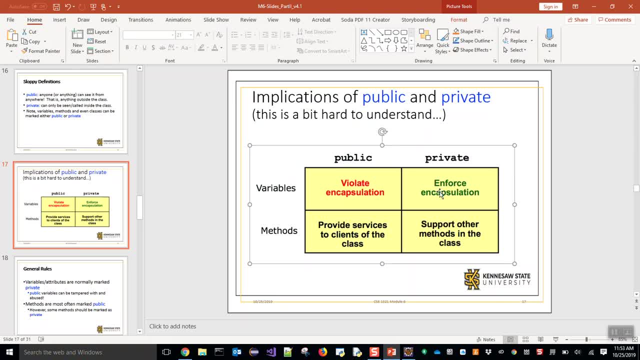 okay so in Cap Mom is one of the peace principles of object-oriented programming okay so in Cap Mom is one of the peace principles of object-oriented programming 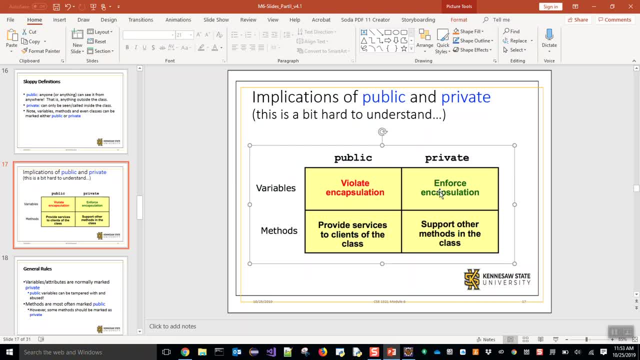 I mean throw is data and objects a data and and methods of a field of study of an object are tied together okay like in a capsule the medicines are tied 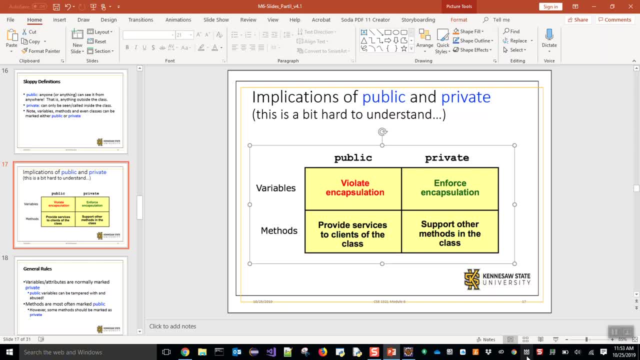 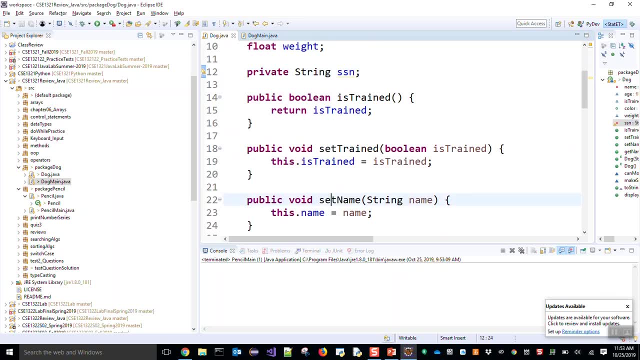 together okay like for instance in our class so what are the data private data these other maybe name and is Gat launch setter try together put together in order to access this okay this is called encapsulation encapsulation is one of 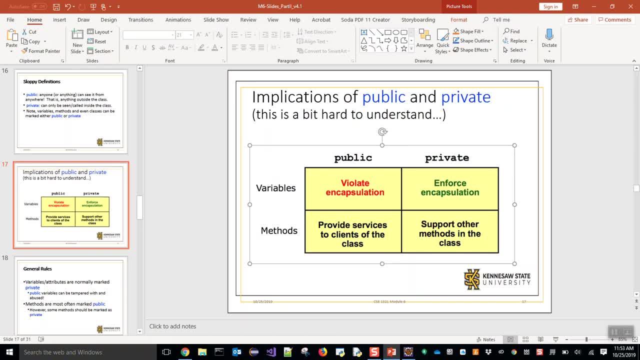 that features of object oriented programming so public and private features can be both variables and methods applicable for both variables and methods okay it can also be this kind 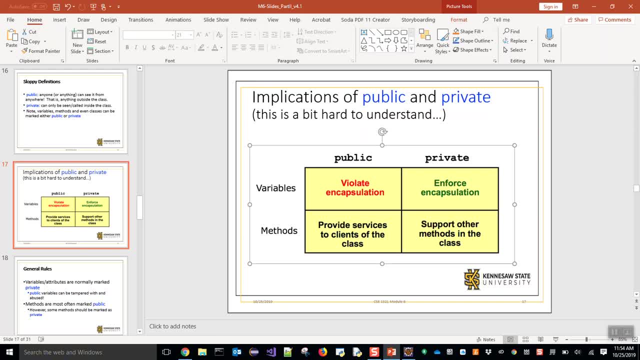 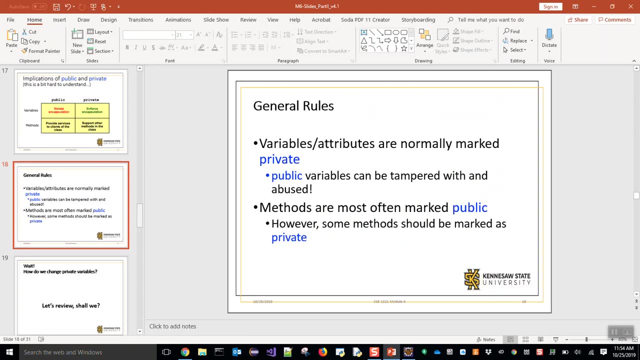 can also be for class if your class is private public then it can be inherited we are not discussing inheritance right now so general rule is that all variables are normally marks should be private should be marked as private but 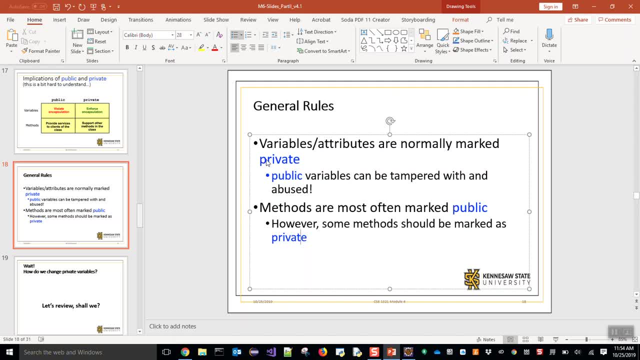 methods should be marked as public and the reason is that if we assign a variable or field or attribute as public then there is a possibility of abuse abuse data is someone from outside can change my that would not like this right so then remember that 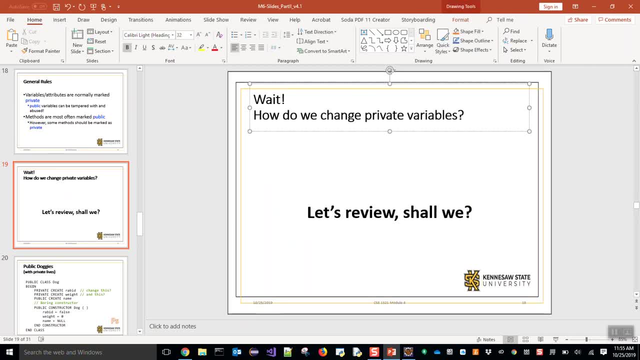 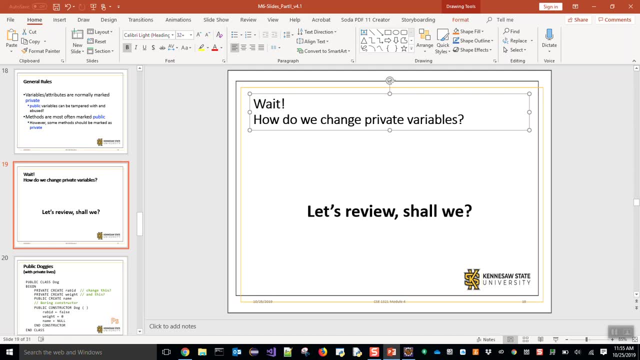 how to use this method how do we change the public private variables by using mutators or modifier 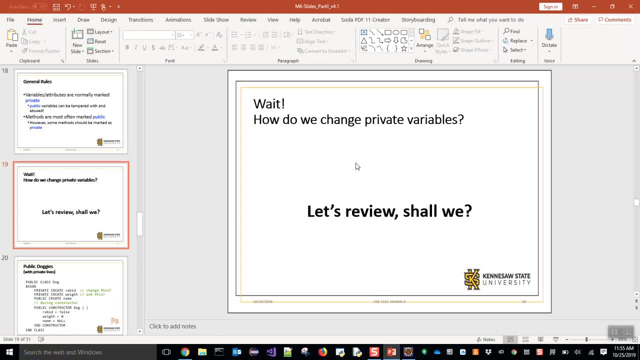 that is called set on method right by calling certain 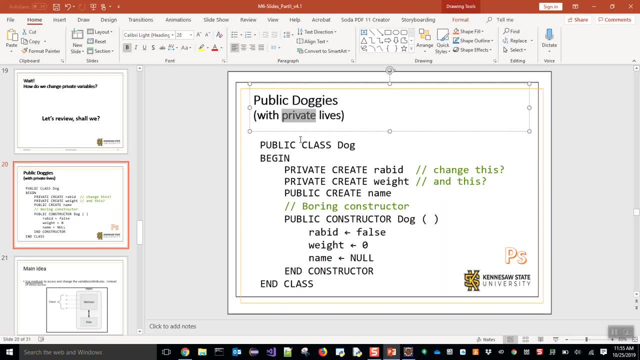 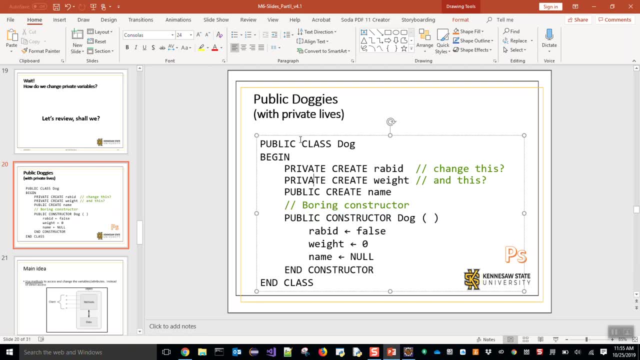 okay here we so this is a classic method where we call an object and see that it contains variables and read our class 10 € 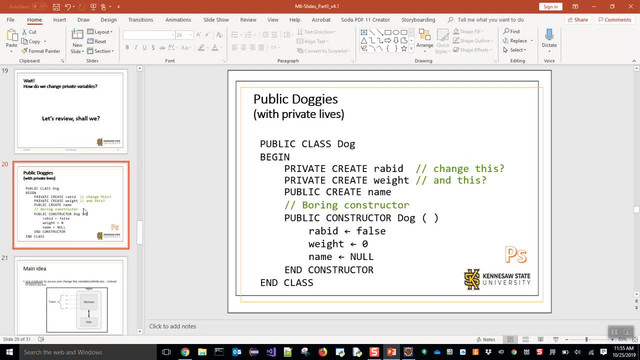 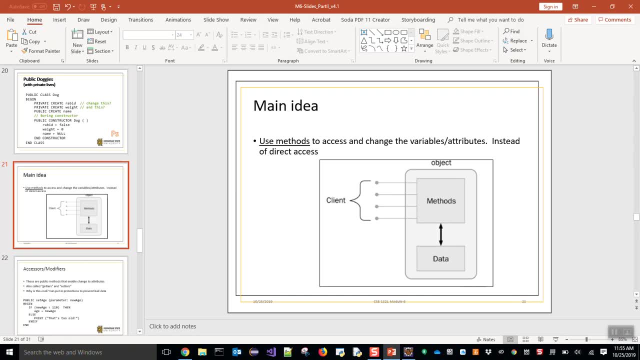 I discussed this in my class that we had some private variables and someual okay so usually what is the concept that again let us review a class that an object is an object contains some variables that holds seven coming from a holds data and an object contains some data and some methods to access those data and when you give a definition of a class we say that a class contains some 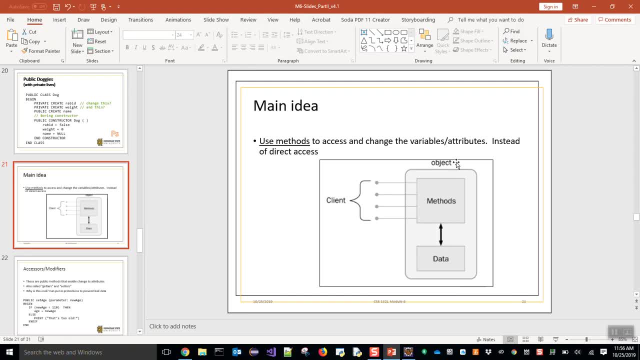 variables and some methods but when you give an object that will tell that an object contains some data not variables okay an object contains some data what kind of data what data that are defined the class of that object so you said remember that everything in this world has a type everything in this world anything has in this world is a type right for instance what is it okay then I asked him what is it right it has a time he said is the market right so everything on if I ask what is it is a watch right it has a type so everything in this world that has a type associated and that type is class okay 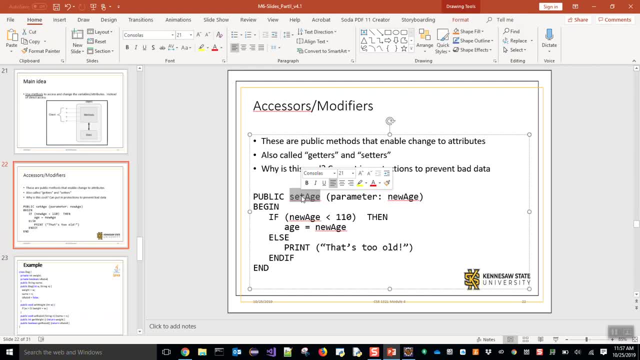 so we discussed access or a modifier that is called this is a setter method the setter method is called okay Sarah is a method over here so with this is method and a method is called a setter method and a method is called a setter method it can have one line of implementation body or it can have multiple lines it can have conditional statement or unconditional statement so 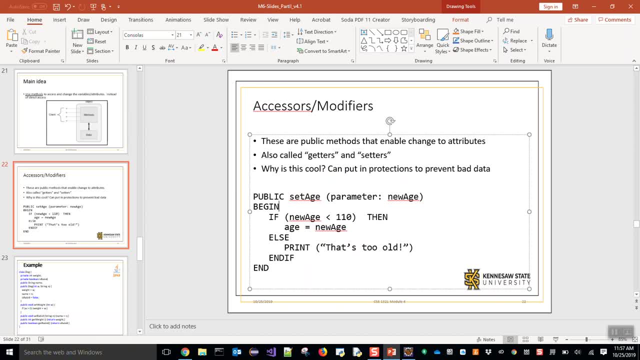 as usual it is a method or a function whatever functions can do a function can do together a setter method can do some time for this error method like there is a conditional statement in order to assign is for instance it is asking if I age is greater than is less than 110 then we are assigning an age but if we ask someone what is your 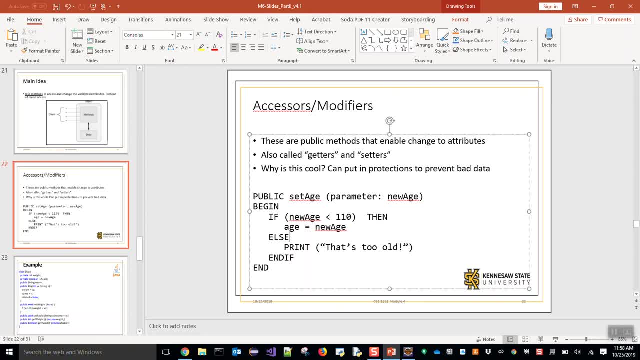 age then it says 120 then we will not believe it then also now you are too old 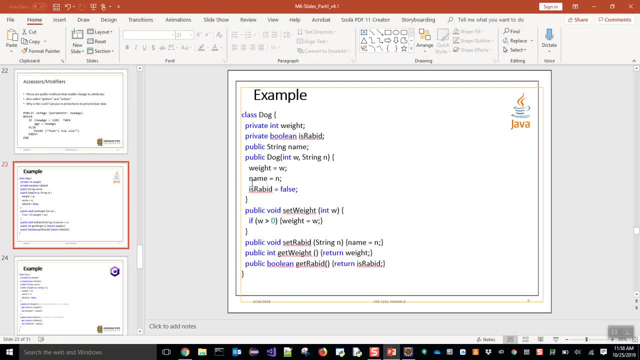 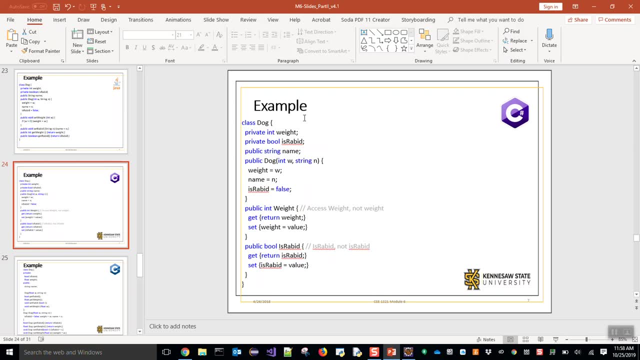 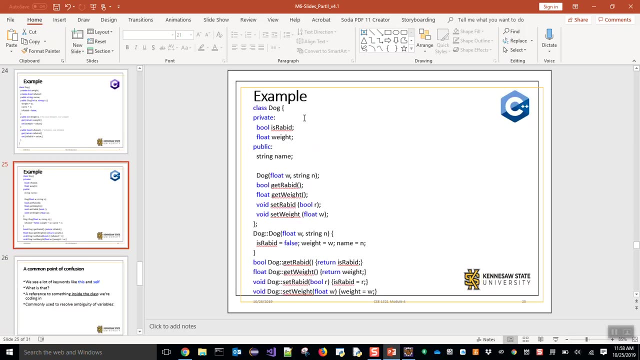 uh so i discussed this how to class define a setter and how to use a greater method but i in my program i had a different field name right it has a different so i like everybody so please do practice for this program and let me know if you get any okay and 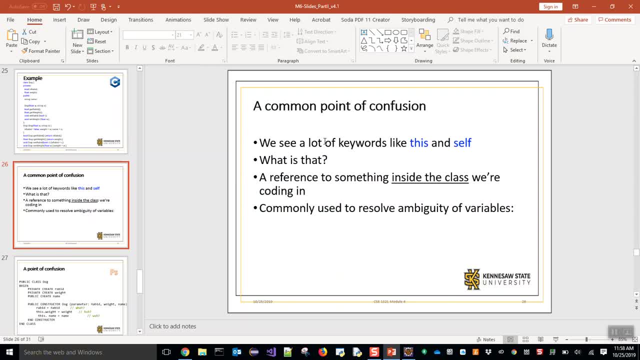 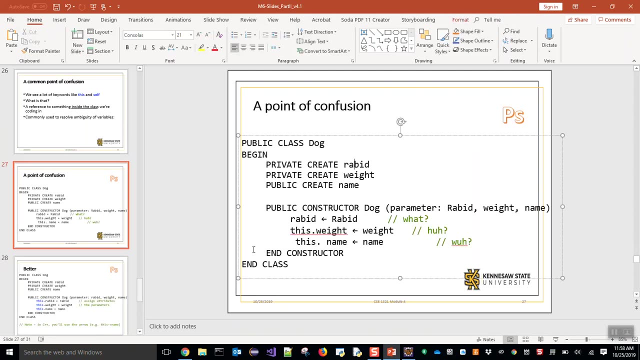 there is a common point of confusion it's called common part of condition we see sometimes you say these were self keyword okay in our programming language python use cell and other programming languages use this keyword i discuss this whenever we have some parameters for any method maybe constructor running method we have a parameter that is exact that has exactly same name of a field name then we use this keyword right for instance here my weight is the same name exactly same name of my weight this is the parameter it has exactly same name of my field name then we assign this dot weight equal to weight 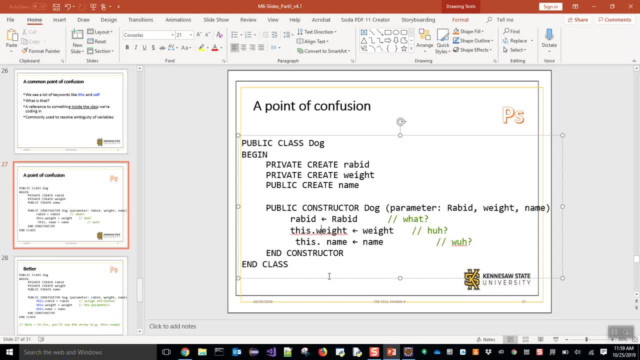 it goes it it goes for object 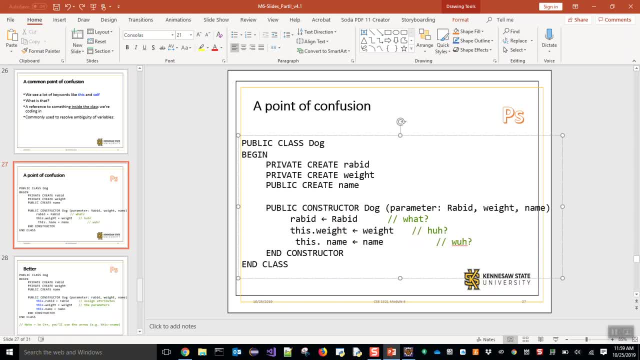 okay so so how does it work let me tell you how does it work so maybe did i do activity 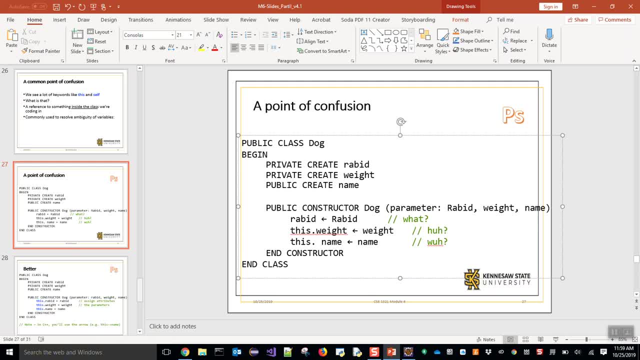 so what is your name and what is your name what is your name 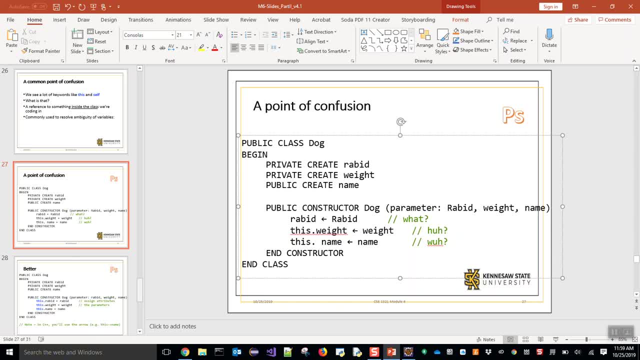 what is your name you see that i asked same question but i got different answer right 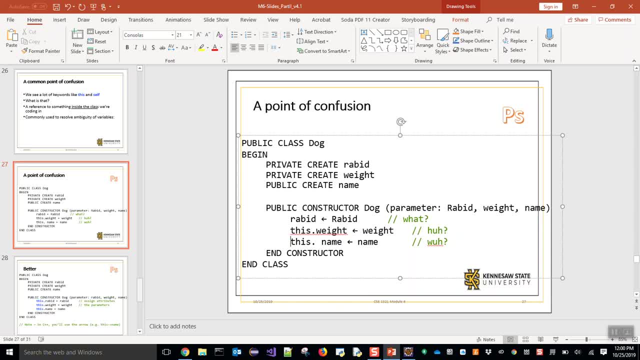 so for that object his name is heart for that object his name is maybe j and another object his name is jackal so that ensures that i say that this dot name equal to name so whatever for this object for this object whatever i will assign when i create him then whatever name i assign for him that will be his name and when i create him whatever name i assigned for him that will be his name so that is ensured by using this keyword 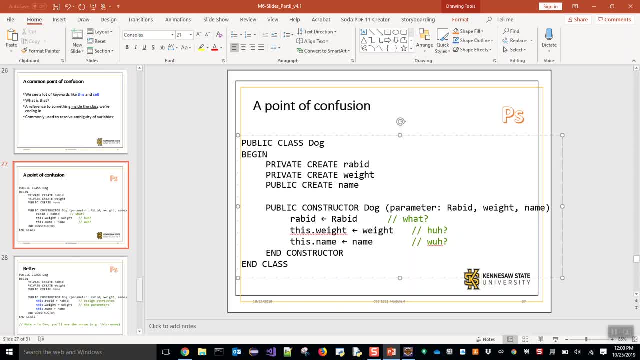 if we will not you do not use this keyword then there is an alternative option that we have to use different name maybe different field name I say can say that name is in uppercase or name in lowercase okay but we people are programmers usually do this is a maybe a challenge for them that may be fun for them they give same 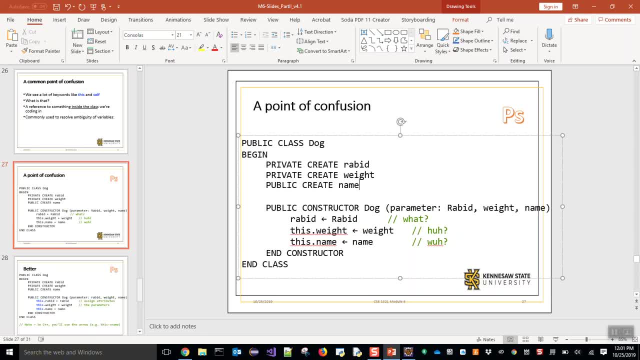 name in your real life maybe we will also do some right for instance we give same name of our child our children name okay maybe John Smith one John Smith two three four we use suffix right in order to distinguish a child from his parent or from his girlfriend we could give different name if we give different first name or last name then we don't need to give suffix right but usually we like to give name as same name 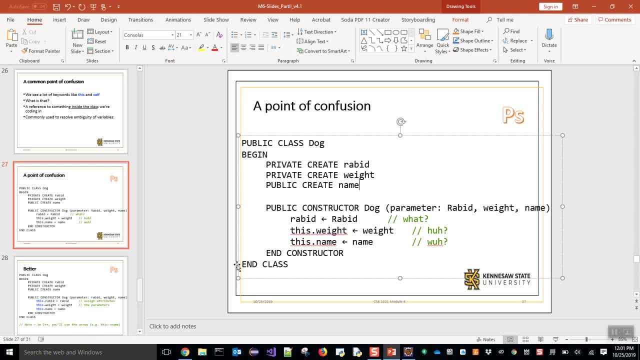 and then you suffix so similar thing 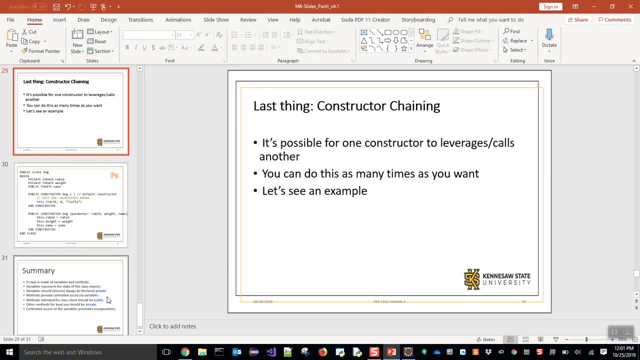 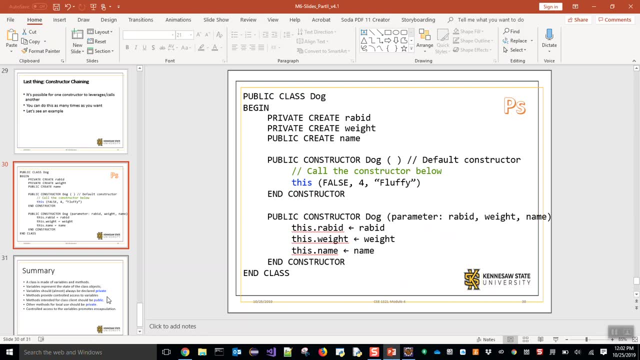 okay constructor chaining is there something actually it is I think may not be applicable for you for introduction but it is here that let us discuss sometime we may need to call one constructor within another constructor that is called constructor chaining for instance here this is the default constructor within this default constructor if I call another constructor this dog constructor then instead of writing this this this dog dog constructor we use this keyword this okay you see that the here this is used as a method this is right right after this so these here this means this 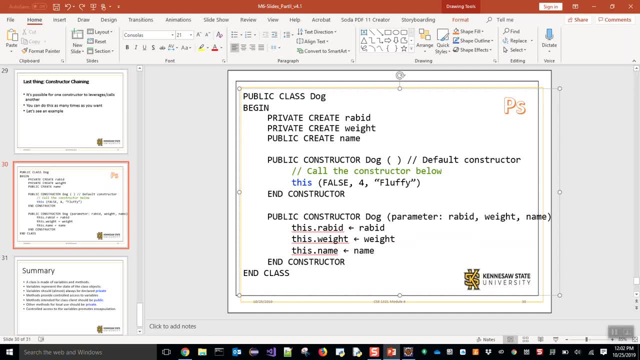 constructor is calling with this value pass for rabbit and for for wait and name for floppy yeah in Java you can do that so I have pseudo code over here so you can code over here in Java it has same name in Java you use this and for some time if we need to call the parent constructor then we use super keyword s-e-p-e-r super keyword 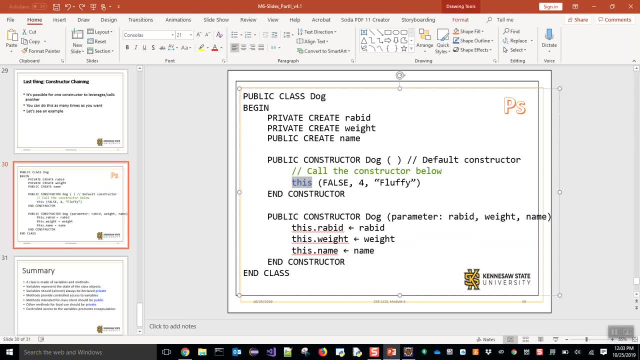 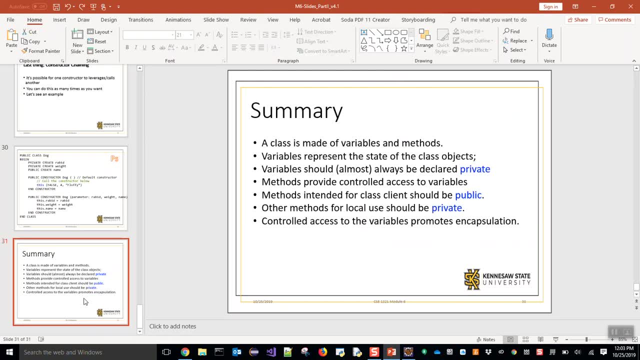 but here maybe we are not going to that kind of in-depth programming so much if you see somewhere you can do you can implement this code i don't have code over here but you can implement 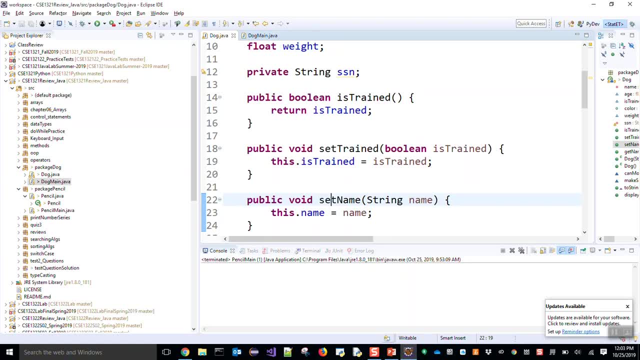 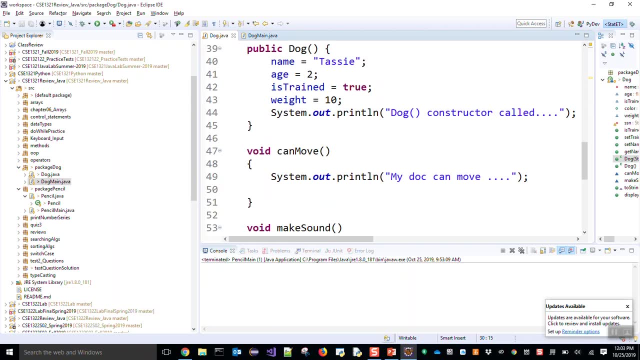 code over here but for instance maybe i can do quickly here i have dog constructor over here right so in my in my what is my empty dog 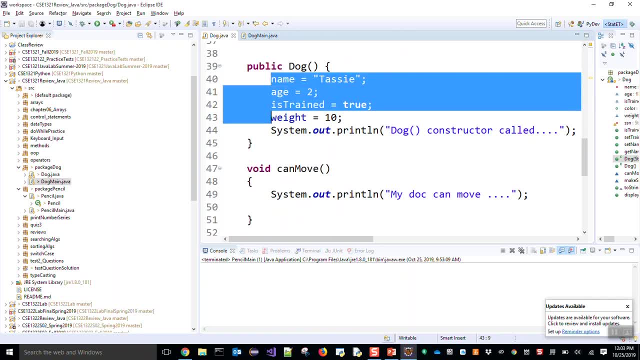 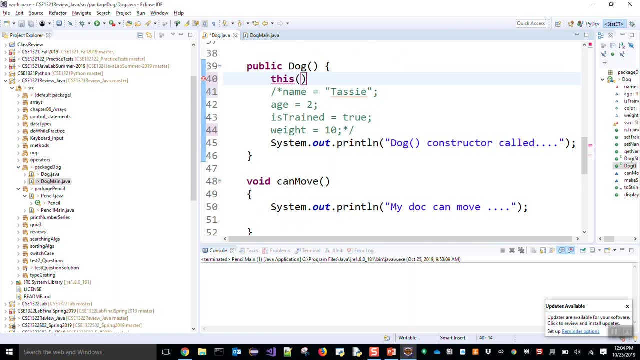 okay here in my i could call this with some values with some name maybe 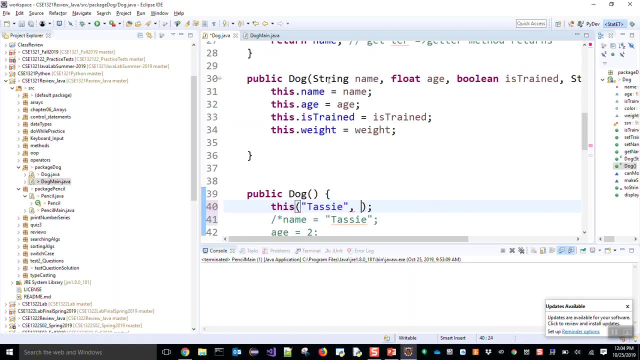 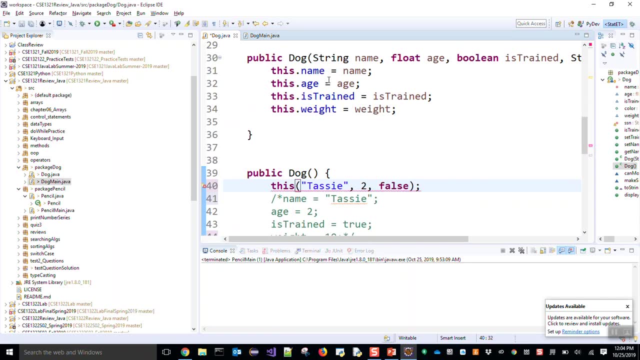 let's see what is my first name name then is maybe two and then boolean is false and what is the next one color 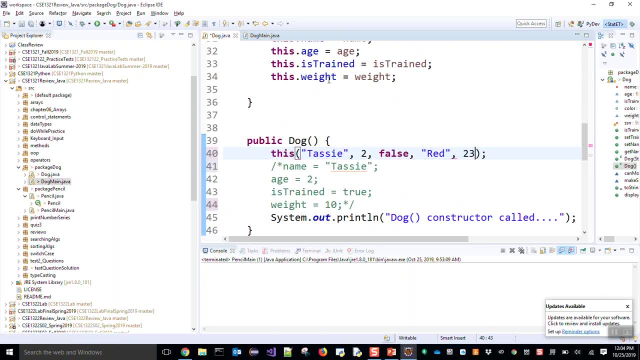 red and what is the weight 23 so this is way so by this way i am calling in my this constructor i am calling this 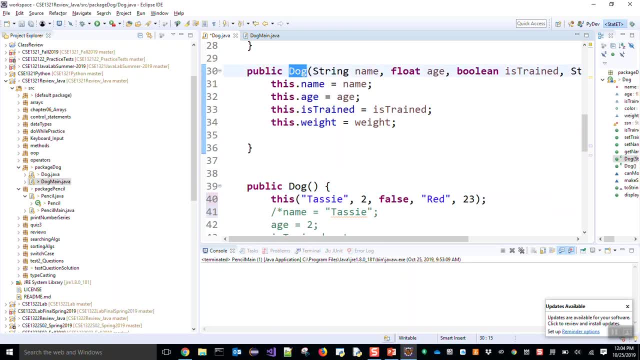 constructor so instead of writing dog over here it will not allow me to write talk i need to use this q1 so this is called on log so this is called 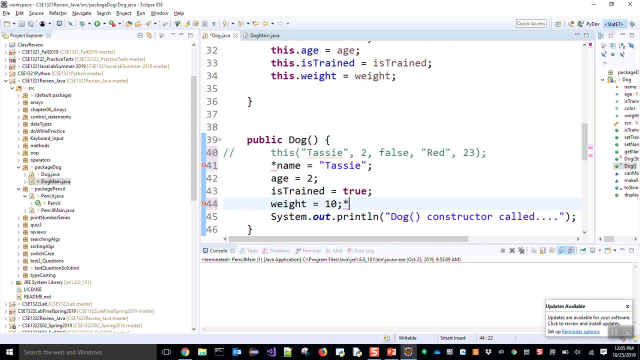 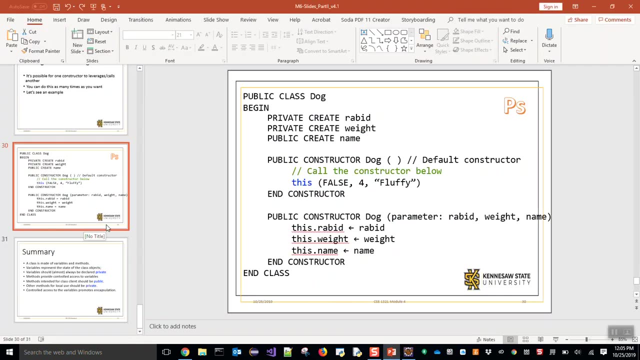 constructor chaining calling one constructor within another constructor 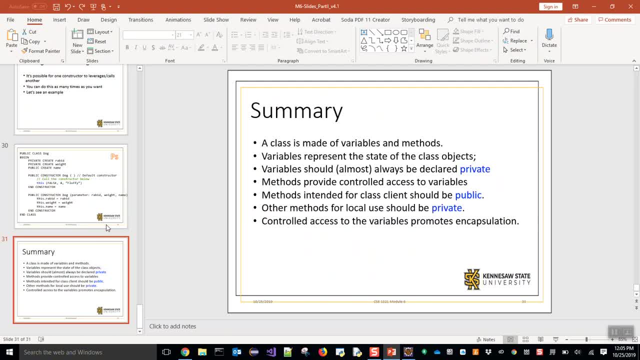 you can do you can practice this one okay and that is the summary whatever so far we have discussed a lot of the things that we need for object oriented programming okay but I have one more thing I want to discuss that is beyond this slice but I think that is important how many minutes I do okay so you know next lecture I will discuss static modified okay I need I need maybe 20 30 25 to 30 minutes then 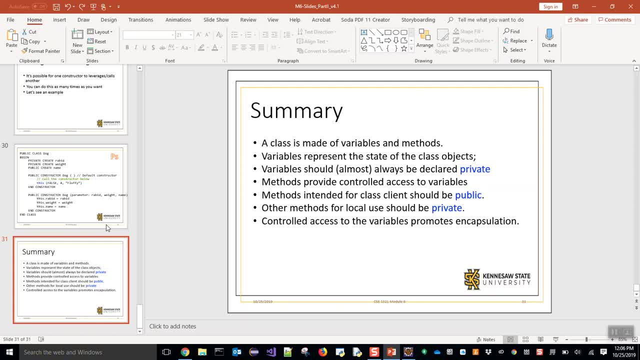 after that we will discuss the world just questions okay anyone has any questions so far no I 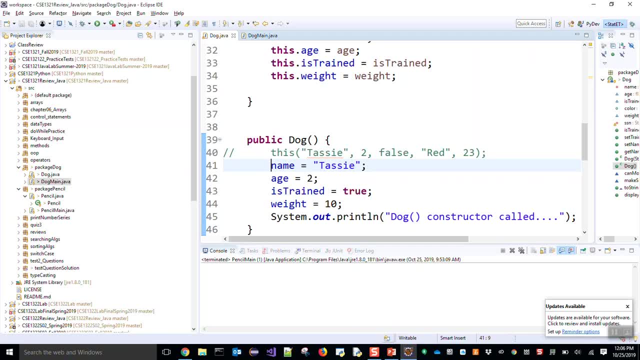 don't use this dot I use this as a as a as a method yes boosting method overriding in the class that is this discredit in the class not in main class 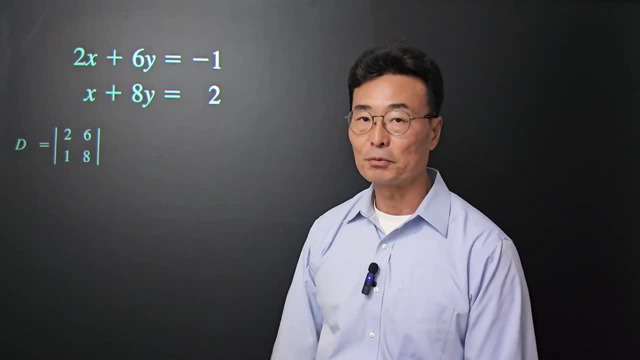 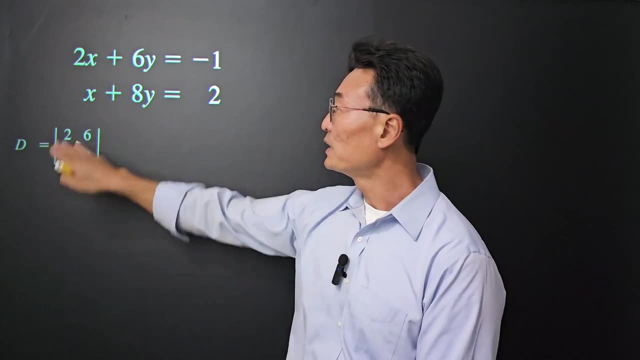 of the matrix of the coefficients of the variables. meaning we take the 2 and the 6 from the x and the y of the first equation, put it on the first row. Next we take the 1 and the 8 from the.